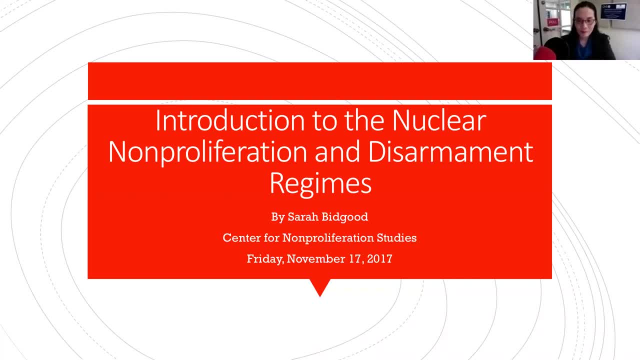 to Sarah. So now, Sarah, you have a microphone. Okay, thank you, Masako, And hello again, everybody. Thank you very much for the opportunity to speak with you today. As Masako indicated, today we're going to be talking about the 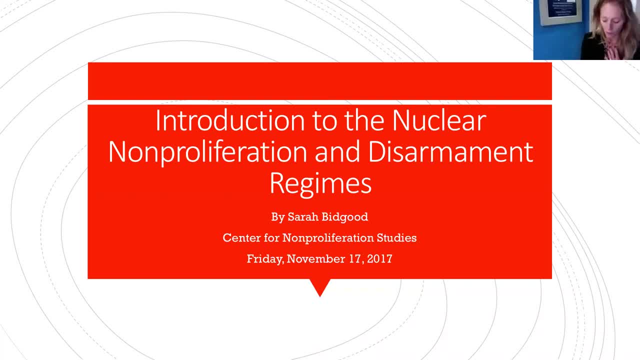 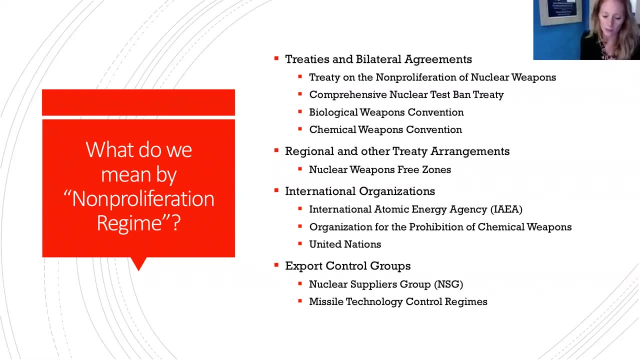 Nuclear Nonproliferation and Disarmament Regimes. So this is just a brief overview of what I hope to cover in today's presentation, but, as always, if you have any questions, please feel free to ask me either now or later. So, in essence, we're going to be talking about several 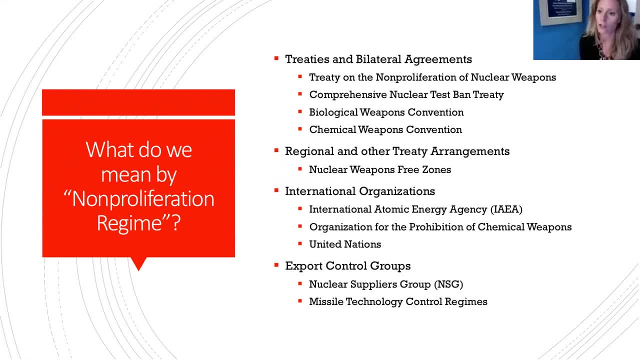 different things which are kind of what we mean by the nonproliferation regime more broadly. Some of these things are treaties and other bilateral agreements. We have regional and other agreements which are things like nuclear weapons free zones etc. We have international organizations, so those are things like the International Atomic Energy Agency or the Organization for the Prohibition of Chemical Weapons. 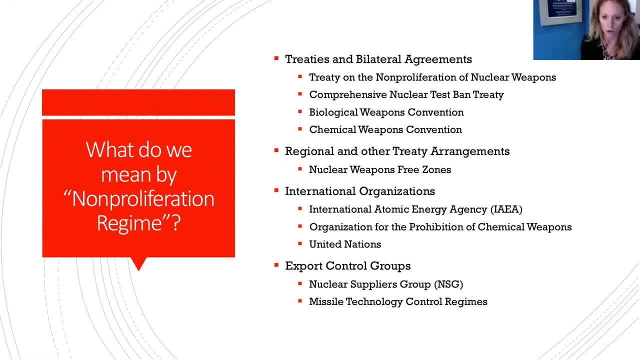 And then we'll briefly touch upon export control groups. So what I'd like to talk about in particular, and kind of the focus of today's talk, is going to be a lot about the NPT, which is the Non-Proliferation Treaty. 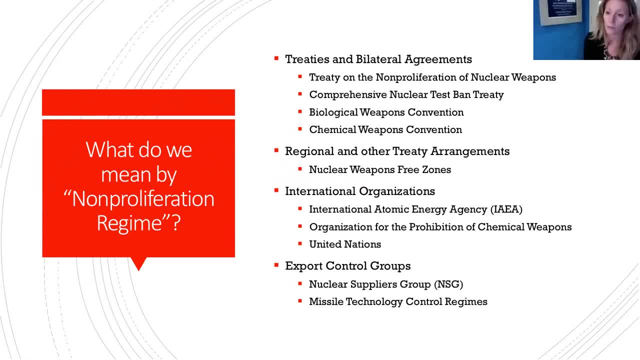 We're also going to talk about the relationship between the International Atomic Energy Agency and the NPT. We'll talk a bit about the new treaty which has been recently negotiated, called the Treaty on the Prohibition of Nuclear Weapons, or the Nuclear Ban Treaty. 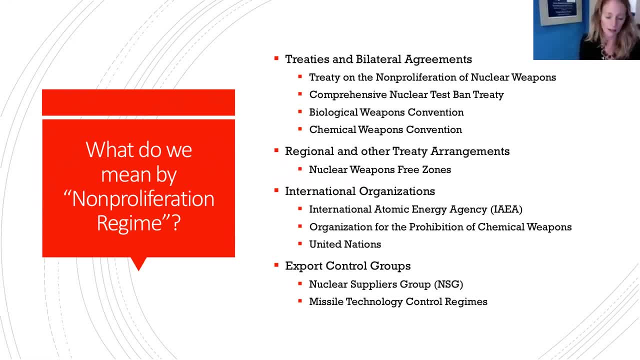 But it's my understanding that you'll have other lectures that delve into that topic more, so I'm not going to focus too much on it, And then we'll also talk about the Biological Weapons Convention, the Chemical Weapons Convention, the Convention on the Prohibition of Nuclear Weapons and the Convention on the Prohibition of Nuclear Weapons. 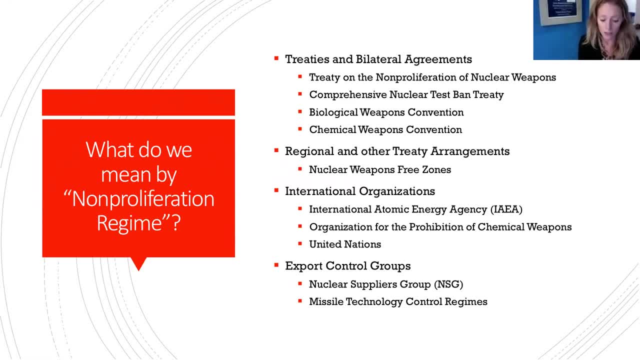 So we'll talk a little bit about that. We'll talk a little bit about the Comprehensive Nuclear Test Ban Treaty, the Conference on Disarmament and, as I said, a little bit about export control regimes towards the end. So one thing that I'd like to say at the outset that I think is helpful for framing this discussion is that when we use the term regime, we mean both sort of documents, things like treaties, negotiating bodies, so conferences and other groups of UN member states who talk about these issues and talk about how to strengthen them. 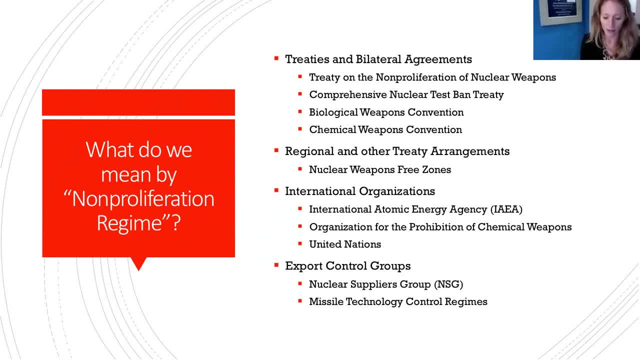 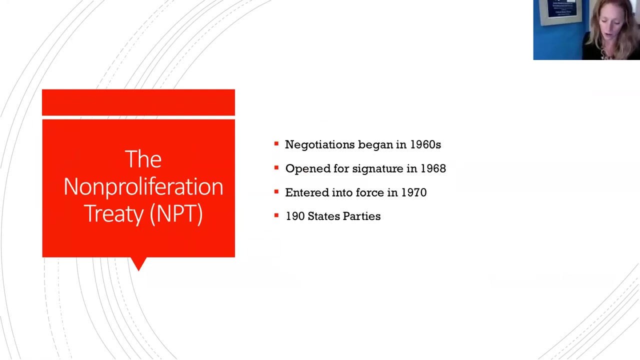 So one thing that I'd like to say at the outset that I think is helpful for framing this discussion is that when we use the term regime, we mean both sort of documents, things like treaties, negotiating bodies, so conferences and other groups of UN member states who talk about these issues and talk about how to strengthen them. 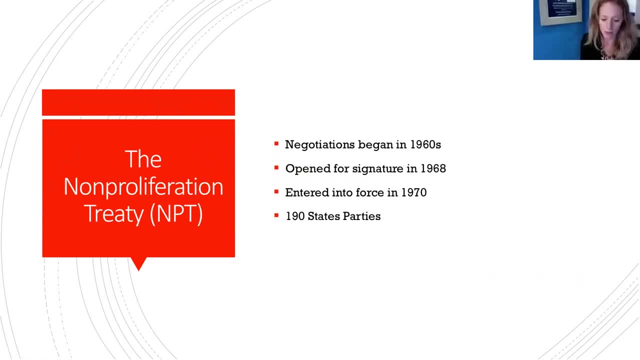 So one thing that I'd like to say at the outset that I think is helpful for framing this discussion is that when we use the term regime, we mean both sort of documents, things like treaties, negotiating bodies, so conferences and other groups of UN member states who talk about these issues and talk about how to strengthen them. 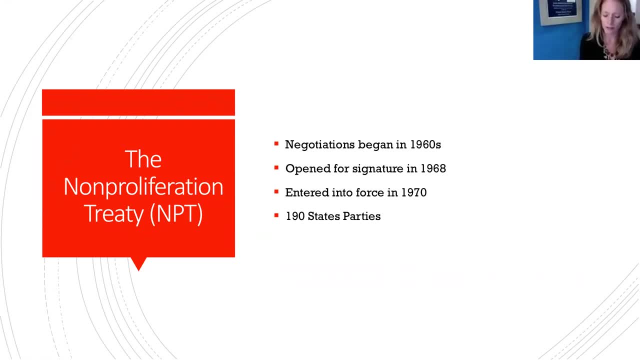 So one thing that I'd like to say at the outset that I think is helpful for framing this discussion is that when we use the term regime, we mean both sort of documents, things like treaties, negotiating bodies, so conferences and other groups of UN member states who talk about these issues and talk about how to strengthen them. 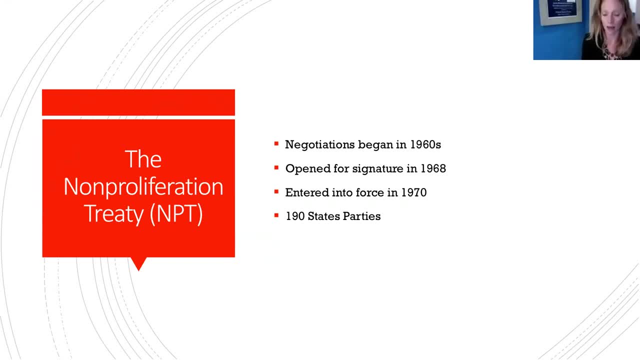 So one thing that I'd like to say at the outset that I think is helpful for framing this discussion is that when we use the term regime, we mean both sort of documents, things like treaties, negotiating bodies, so conferences and other groups of UN member states who talk about these issues and talk about how to strengthen them. 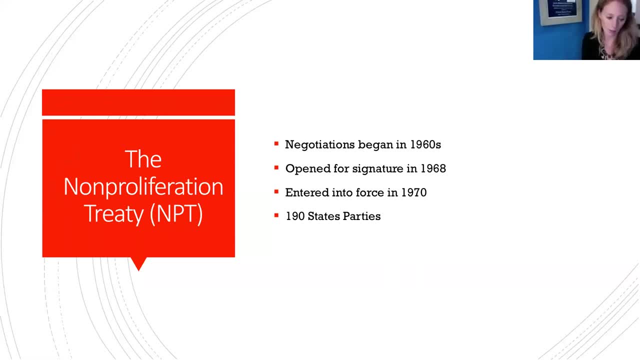 So one thing that I'd like to say at the outset that I think is helpful for framing this discussion is that when we use the term regime, we mean both sort of documents, things like treaties, negotiating bodies, so conferences and other groups of UN member states who talk about these issues and talk about how to strengthen them. 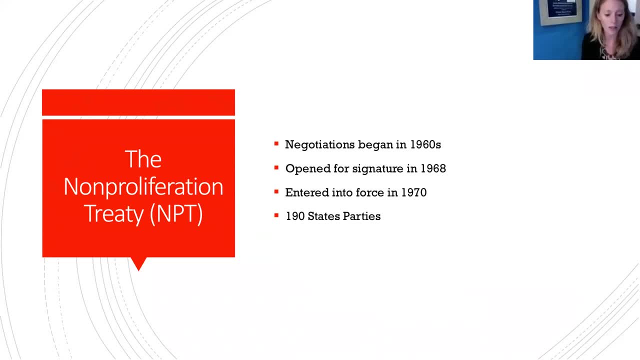 So one thing that I'd like to say at the outset that I think is helpful for framing this discussion is that when we use the term regime, we mean both sort of documents, things like treaties, negotiating bodies, so conferences and other groups of UN member states who talk about these issues and talk about how to strengthen them. 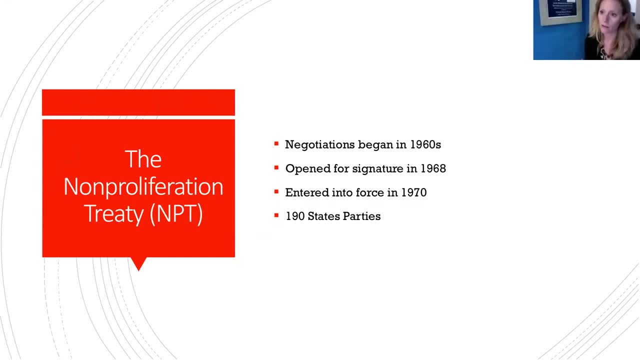 So one thing that I'd like to say at the outset that I think is helpful for framing this discussion is that when we use the term regime, we mean both sort of documents, things like treaties, negotiating bodies, so conferences and other groups of UN member states who talk about these issues and talk about how to strengthen them. 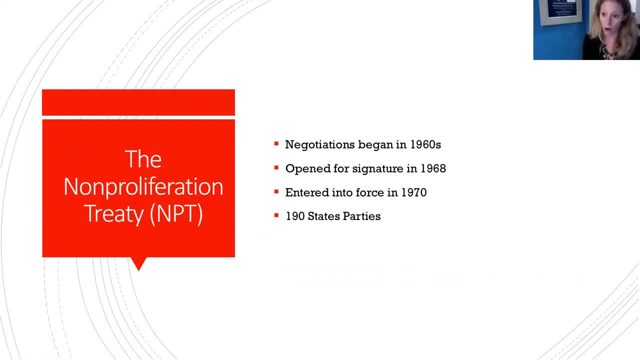 So one thing that I'd like to say at the outset that I think is helpful for framing this discussion is that when we use the term regime, we mean both sort of documents, things like treaties, negotiating bodies, so conferences and other groups of UN member states who talk about these issues and talk about how to strengthen them. 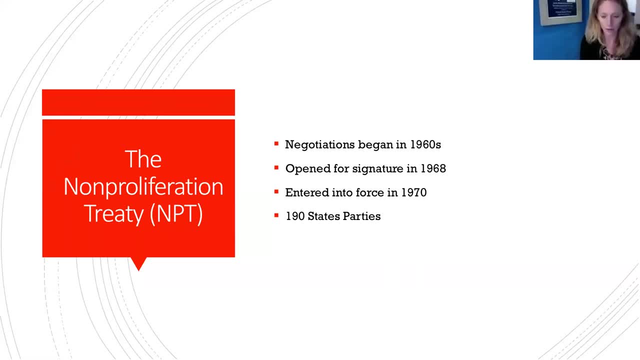 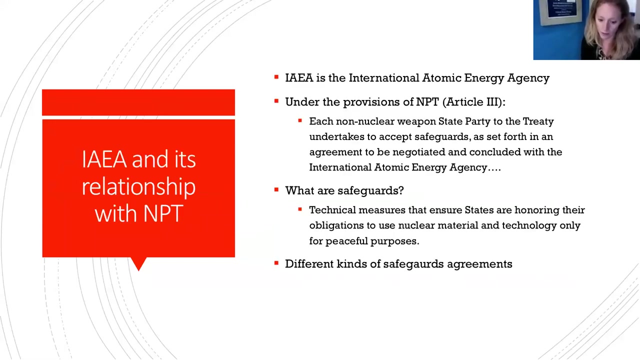 So one thing that I'd like to say at the outset that I think is helpful for framing this discussion is that when we use the term regime, we mean both sort of documents, things like treaties, negotiating bodies, so conferences and other groups of UN member states who talk about these issues and talk about how to strengthen them. 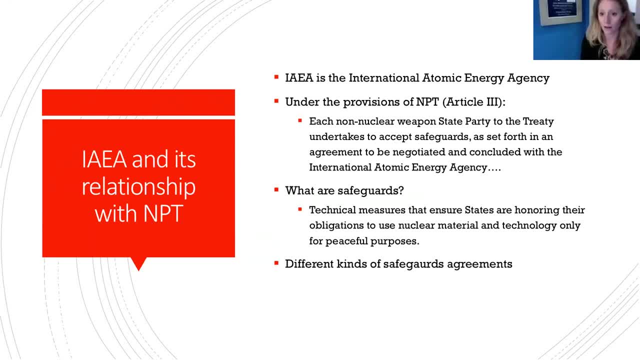 So one thing that I'd like to say at the outset that I think is helpful for framing this discussion is that when we use the term regime, we mean both sort of documents, things like treaties, negotiating bodies, so conferences and other groups of UN member states who talk about these issues and talk about how to strengthen them. 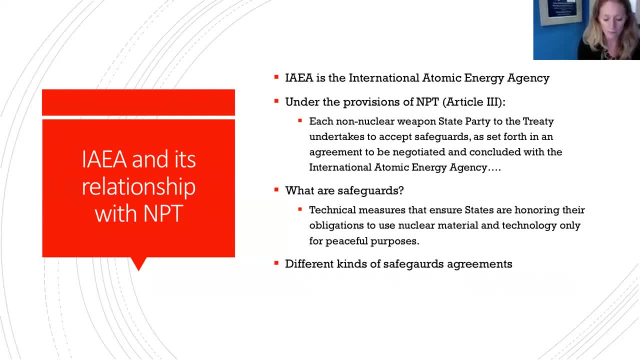 So one thing that I'd like to say at the outset that I think is helpful for framing this discussion is that when we use the term regime, we mean both sort of documents, things like treaties, negotiating bodies, so conferences and other groups of UN member states who talk about these issues and talk about how to strengthen them. 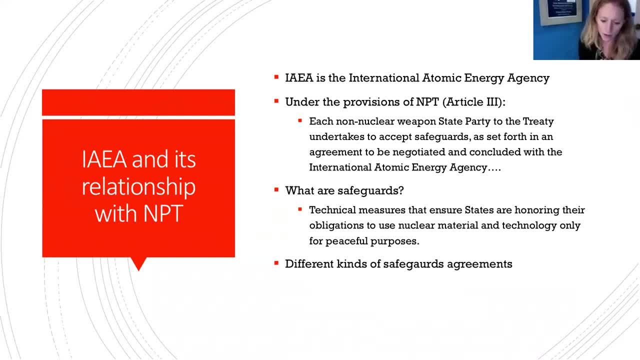 So one thing that I'd like to say at the outset that I think is helpful for framing this discussion is that when we use the term regime, we mean both sort of documents, things like treaties, negotiating bodies, so conferences and other groups of UN member states who talk about these issues and talk about how to strengthen them. 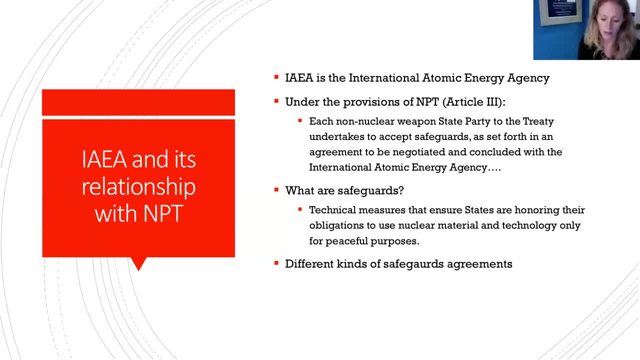 So one thing that I'd like to say at the outset that I think is helpful for framing this discussion is that when we use the term regime, we mean both sort of documents, things like treaties, negotiating bodies, so conferences and other groups of UN member states who talk about these issues and talk about how to strengthen them. 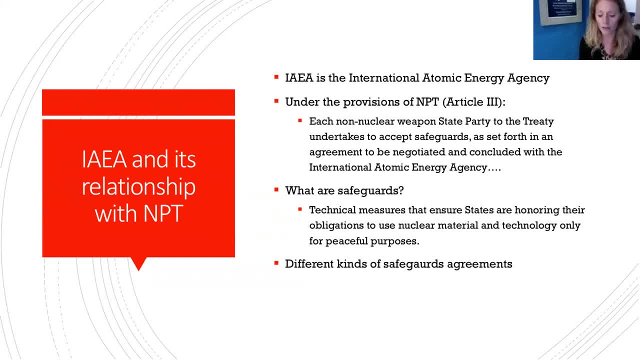 So one thing that I'd like to say at the outset that I think is helpful for framing this discussion is that when we use the term regime, we mean both sort of documents, things like treaties, negotiating bodies, so conferences and other groups of UN member states who talk about these issues and talk about how to strengthen them. 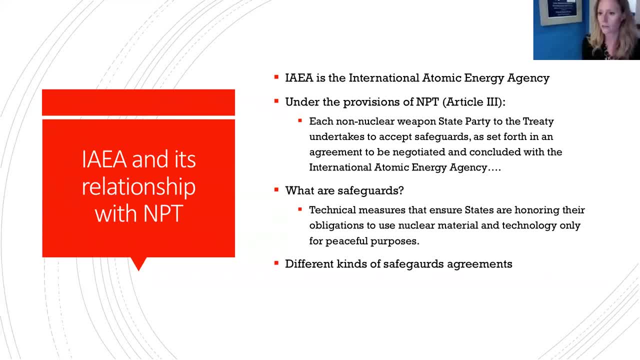 So one thing that I'd like to say at the outset that I think is helpful for framing this discussion is that when we use the term regime, we mean both sort of documents, things like treaties, negotiating bodies, so conferences and other groups of UN member states who talk about these issues and talk about how to strengthen them. 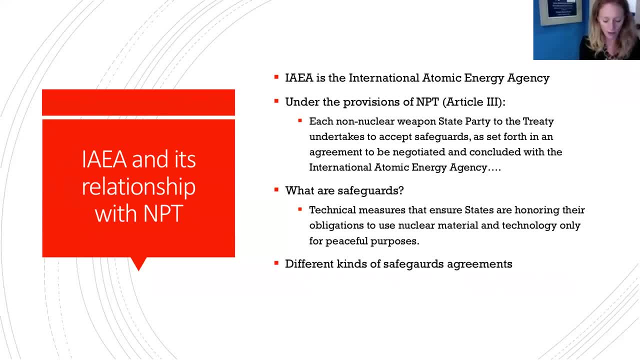 So one thing that I'd like to say at the outset that I think is helpful for framing this discussion is that when we use the term regime, we mean both sort of documents, things like treaties, negotiating bodies, so conferences and other groups of UN member states who talk about these issues and talk about how to strengthen them. 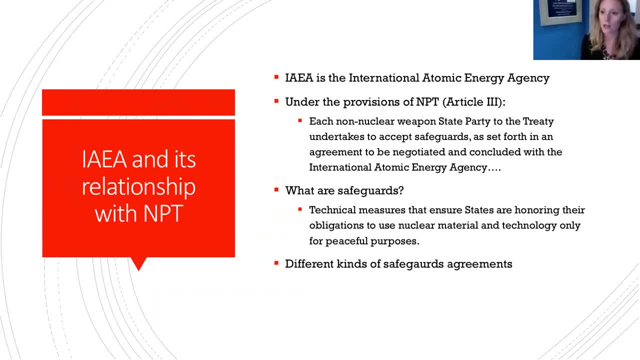 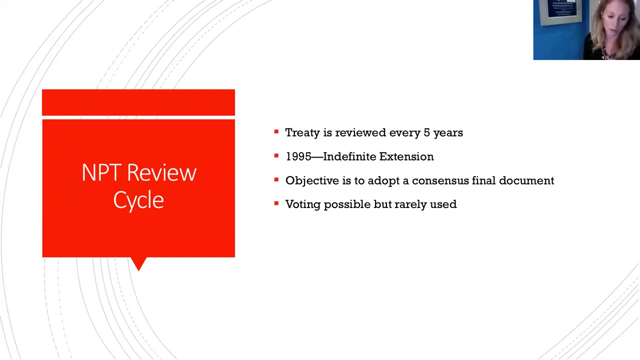 So one thing that I'd like to say at the outset that I think is helpful for framing this discussion is that when we use the term regime, we mean both sort of documents, things like treaties, negotiating bodies, so conferences and other groups of UN member states who talk about these issues and talk about how to strengthen them. 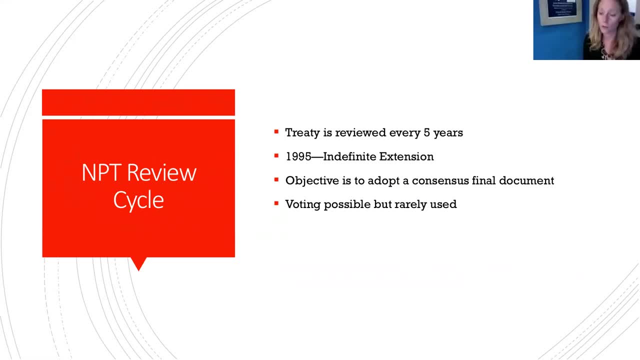 So one thing that I'd like to say at the outset that I think is helpful for framing this discussion is that when we use the term regime, we mean both sort of documents, things like treaties, negotiating bodies, so conferences and other groups of UN member states who talk about these issues and talk about how to strengthen them. 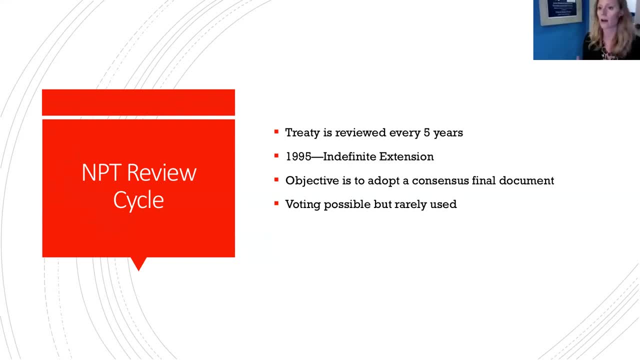 So one thing that I'd like to say at the outset that I think is helpful for framing this discussion is that when we use the term regime, we mean both sort of documents, things like treaties, negotiating bodies, so conferences and other groups of UN member states who talk about these issues and talk about how to strengthen them. 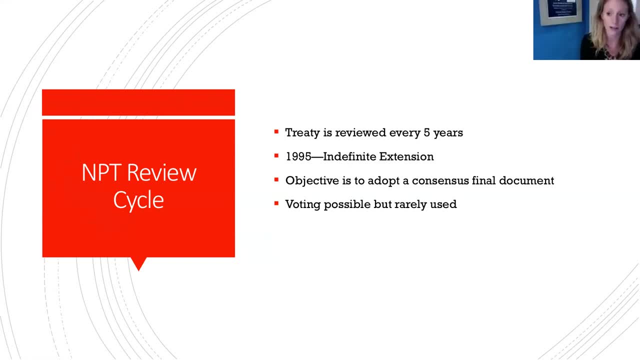 So one thing that I'd like to say at the outset that I think is helpful for framing this discussion is that when we use the term regime, we mean both sort of documents, things like treaties, negotiating bodies, so conferences and other groups of UN member states who talk about these issues and talk about how to strengthen them. 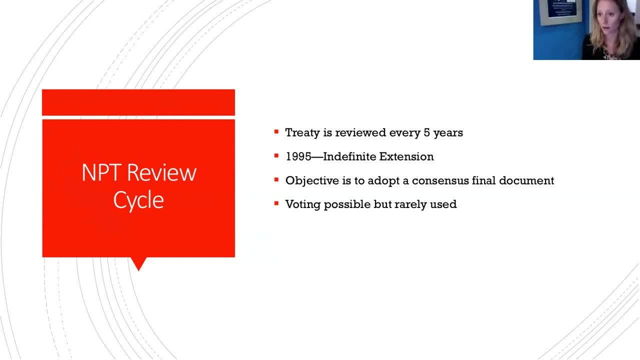 So one thing that I'd like to say at the outset that I think is helpful for framing this discussion is that when we use the term regime, we mean both sort of documents, things like treaties, negotiating bodies, so conferences and other groups of UN member states who talk about these issues and talk about how to strengthen them. 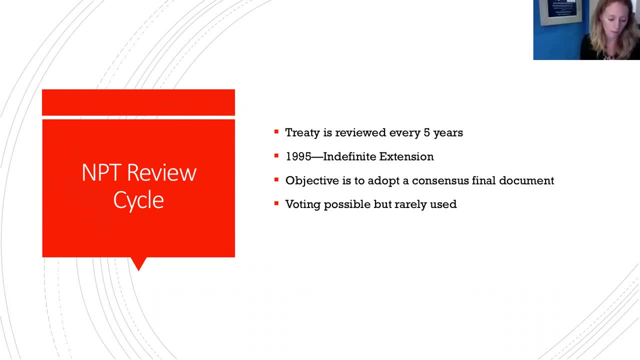 So one thing that I'd like to say at the outset that I think is helpful for framing this discussion is that when we use the term regime, we mean both sort of documents, things like treaties, negotiating bodies, so conferences and other groups of UN member states who talk about these issues and talk about how to strengthen them. 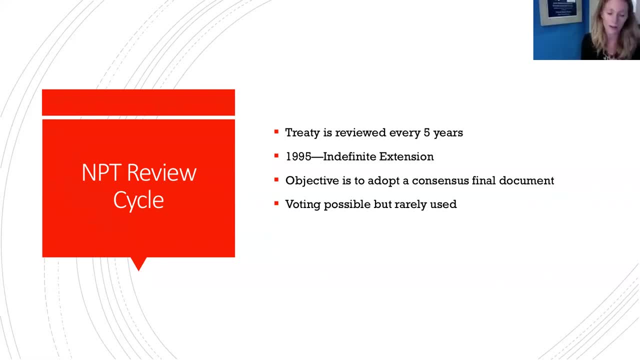 So one thing that I'd like to say at the outset that I think is helpful for framing this discussion is that when we use the term regime, we mean both sort of documents, things like treaties, negotiating bodies, so conferences and other groups of UN member states who talk about these issues and talk about how to strengthen them. 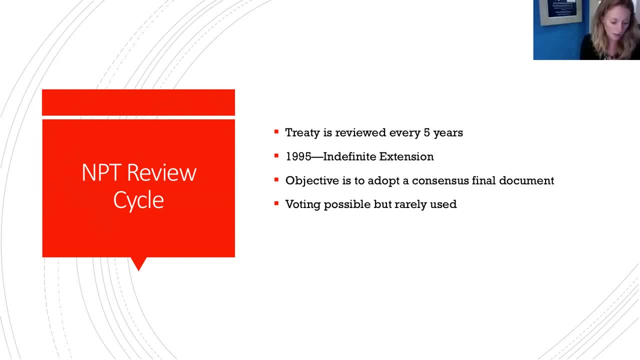 So one thing that I'd like to say at the outset that I think is helpful for framing this discussion is that when we use the term regime, we mean both sort of documents, things like treaties, negotiating bodies, so conferences and other groups of UN member states who talk about these issues and talk about how to strengthen them. 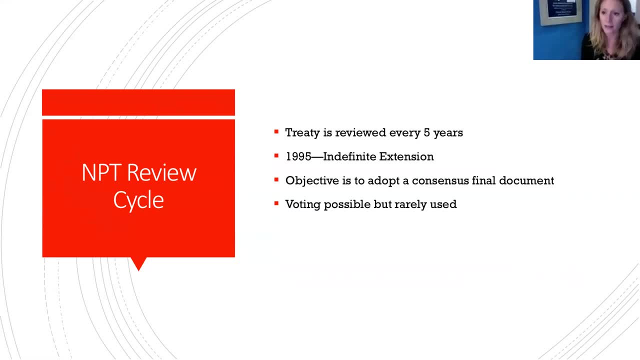 So one thing that I'd like to say at the outset that I think is helpful for framing this discussion is that when we use the term regime, we mean both sort of documents, things like treaties, negotiating bodies, so conferences and other groups of UN member states who talk about these issues and talk about how to strengthen them. 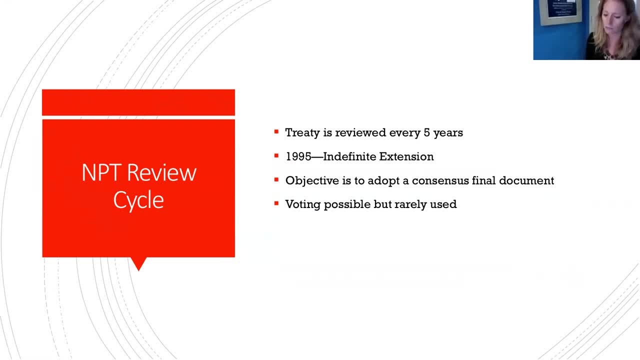 So one thing that I'd like to say at the outset that I think is helpful for framing this discussion is that when we use the term regime, we mean both sort of documents, things like treaties, negotiating bodies, so conferences and other groups of UN member states who talk about these issues and talk about how to strengthen them. 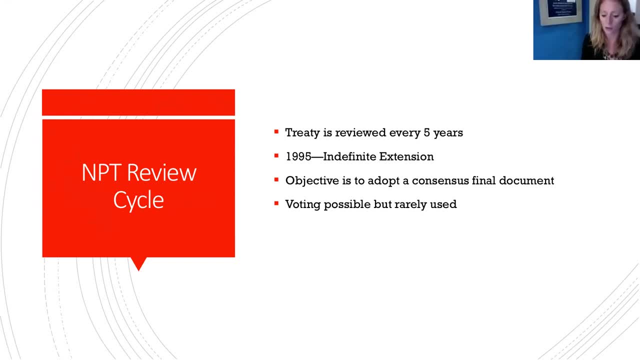 So one thing that I'd like to say at the outset that I think is helpful for framing this discussion is that when we use the term regime, we mean both sort of documents, things like treaties, negotiating bodies, so conferences and other groups of UN member states who talk about these issues and talk about how to strengthen them. 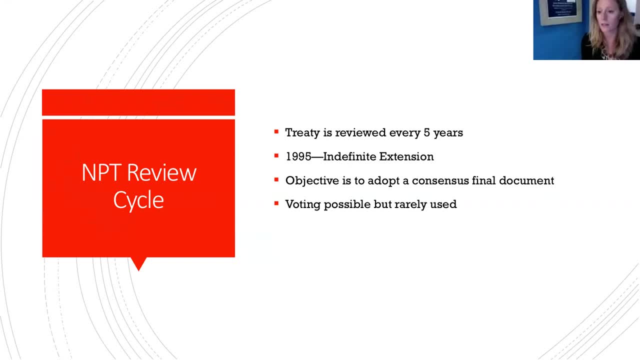 So one thing that I'd like to say at the outset that I think is helpful for framing this discussion is that when we use the term regime, we mean both sort of documents, things like treaties, negotiating bodies, so conferences and other groups of UN member states who talk about these issues and talk about how to strengthen them. 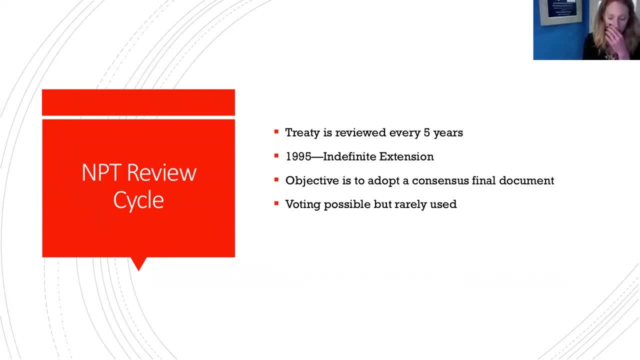 So one thing that I'd like to say at the outset that I think is helpful for framing this discussion is that when we use the term regime, we mean both sort of documents, things like treaties, negotiating bodies, so conferences and other groups of UN member states who talk about these issues and talk about how to strengthen them. 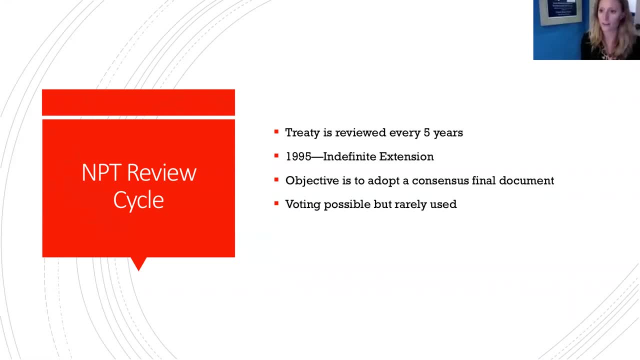 So one thing that I'd like to say at the outset that I think is helpful for framing this discussion is that when we use the term regime, we mean both sort of documents, things like treaties, negotiating bodies, so conferences and other groups of UN member states who talk about these issues and talk about how to strengthen them. 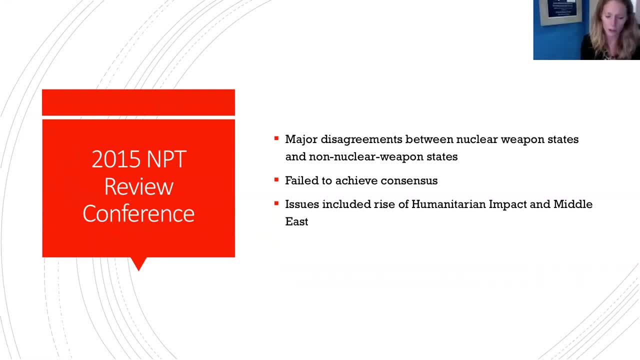 So one thing that I'd like to say at the outset that I think is helpful for framing this discussion is that when we use the term regime, we mean both sort of documents, things like treaties, negotiating bodies, so conferences and other groups of UN member states who talk about these issues and talk about how to strengthen them. 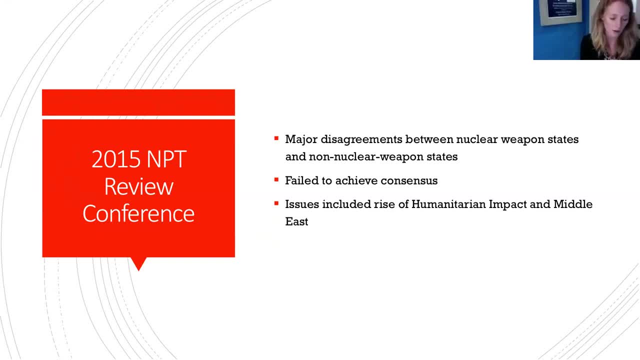 So one thing that I'd like to say at the outset that I think is helpful for framing this discussion is that when we use the term regime, we mean both sort of documents, things like treaties, negotiating bodies, so conferences and other groups of UN member states who talk about these issues and talk about how to strengthen them. 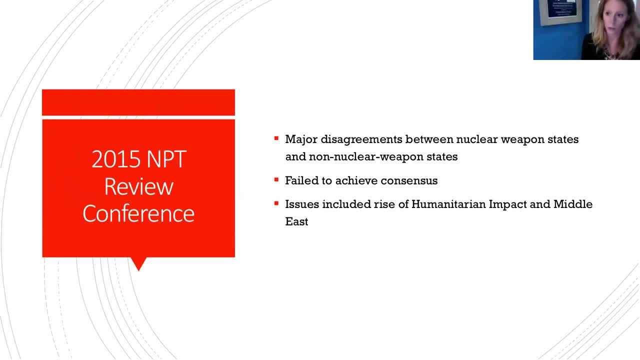 So one thing that I'd like to say at the outset that I think is helpful for framing this discussion is that when we use the term regime, we mean both sort of documents, things like treaties, negotiating bodies, so conferences and other groups of UN member states who talk about these issues and talk about how to strengthen them. 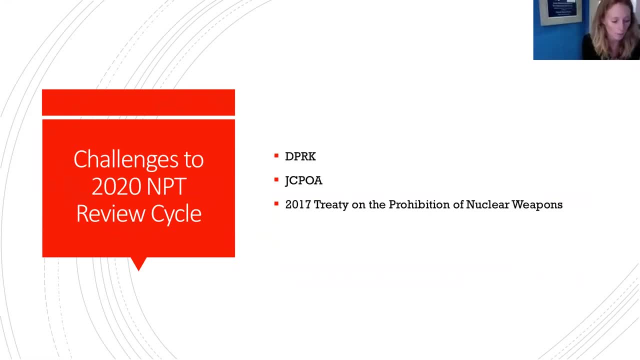 So one thing that I'd like to say at the outset that I think is helpful for framing this discussion is that when we use the term regime, we mean both sort of documents, things like treaties, negotiating bodies, so conferences and other groups of UN member states who talk about these issues and talk about how to strengthen them. 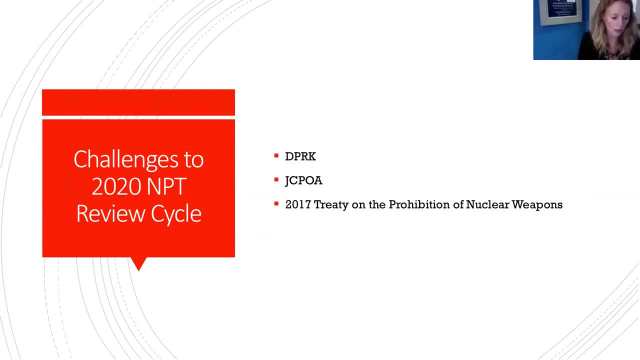 So one thing that I'd like to say at the outset that I think is helpful for framing this discussion is that when we use the term regime, we mean both sort of documents, things like treaties, negotiating bodies, so conferences and other groups of UN member states who talk about these issues and talk about how to strengthen them. 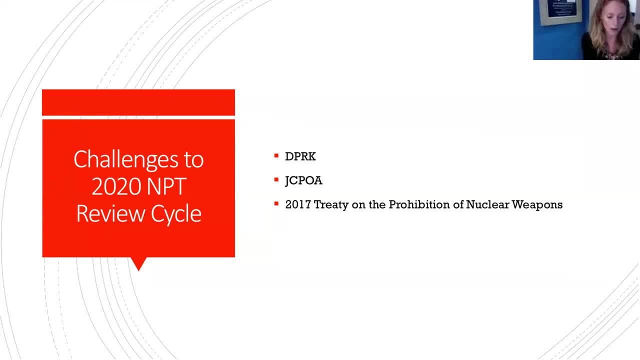 So one thing that I'd like to say at the outset that I think is helpful for framing this discussion is that when we use the term regime, we mean both sort of documents, things like treaties, negotiating bodies, so conferences and other groups of UN member states who talk about these issues and talk about how to strengthen them. 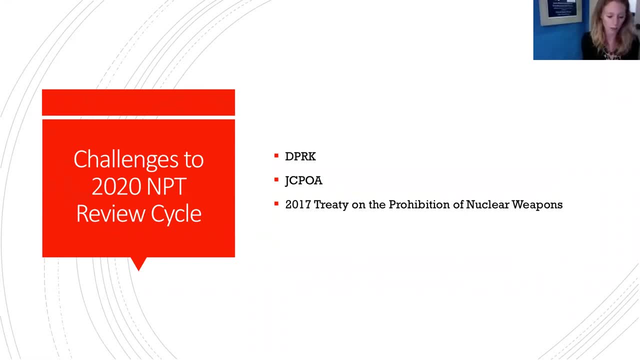 So one thing that I'd like to say at the outset that I think is helpful for framing this discussion is that when we use the term regime, we mean both sort of documents, things like treaties, negotiating bodies, so conferences and other groups of UN member states who talk about these issues and talk about how to strengthen them. 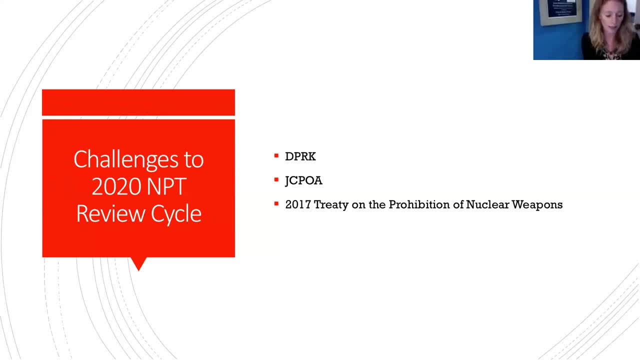 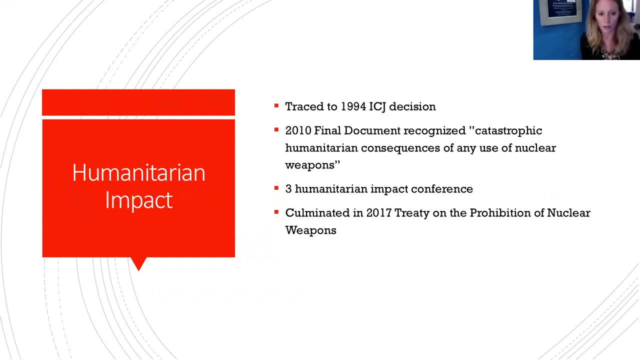 So one thing that I'd like to say at the outset that I think is helpful for framing this discussion is that when we use the term regime, we mean both sort of documents, things like treaties, negotiating bodies, so conferences and other groups of UN member states who talk about these issues and talk about how to strengthen them. 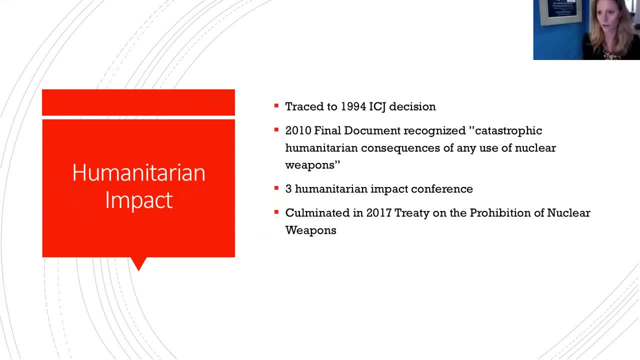 So one thing that I'd like to say at the outset that I think is helpful for framing this discussion is that when we use the term regime, we mean both sort of documents, things like treaties, negotiating bodies, so conferences and other groups of UN member states who talk about these issues and talk about how to strengthen them. 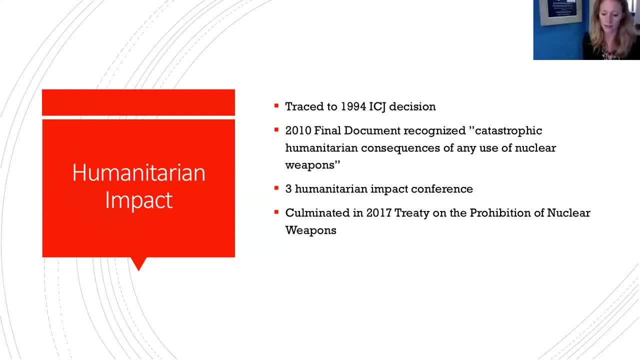 So one thing that I'd like to say at the outset that I think is helpful for framing this discussion is that when we use the term regime, we mean both sort of documents, things like treaties, negotiating bodies, so conferences and other groups of UN member states who talk about these issues and talk about how to strengthen them. 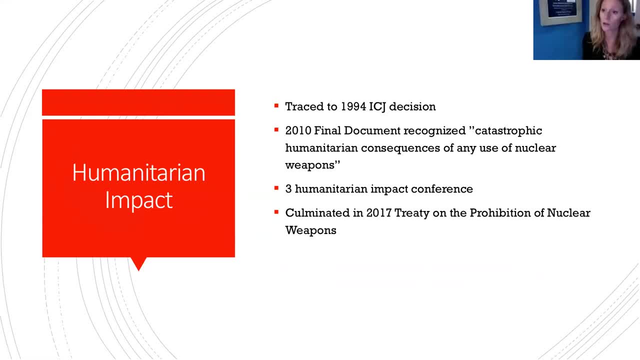 So one thing that I'd like to say at the outset that I think is helpful for framing this discussion is that when we use the term regime, we mean both sort of documents, things like treaties, negotiating bodies, so conferences and other groups of UN member states who talk about these issues and talk about how to strengthen them. 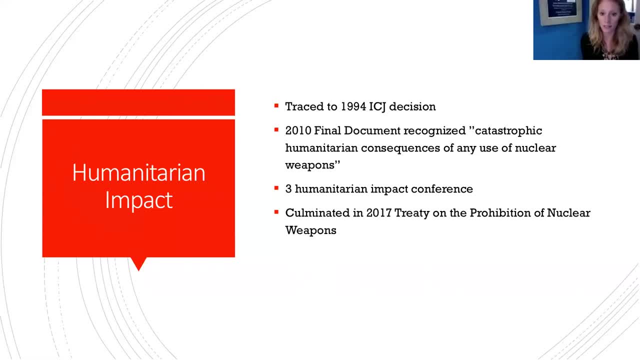 So one thing that I'd like to say at the outset that I think is helpful for framing this discussion is that when we use the term regime, we mean both sort of documents, things like treaties, negotiating bodies, so conferences and other groups of UN member states who talk about these issues and talk about how to strengthen them. 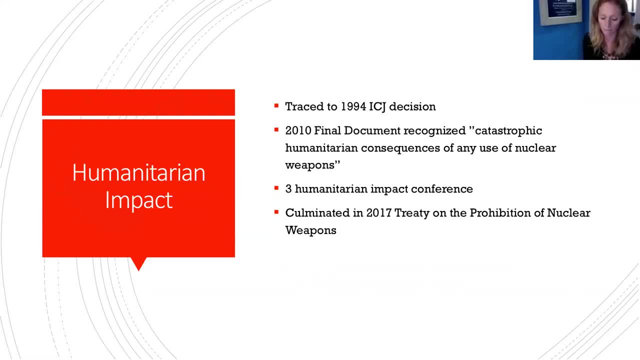 So one thing that I'd like to say at the outset that I think is helpful for framing this discussion is that when we use the term regime, we mean both sort of documents, things like treaties, negotiating bodies, so conferences and other groups of UN member states who talk about these issues and talk about how to strengthen them. 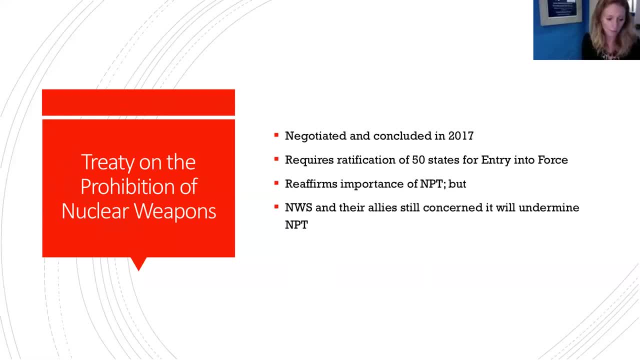 So one thing that I'd like to say at the outset that I think is helpful for framing this discussion is that when we use the term regime, we mean both sort of documents, things like treaties, negotiating bodies, so conferences and other groups of UN member states who talk about these issues and talk about how to strengthen them. 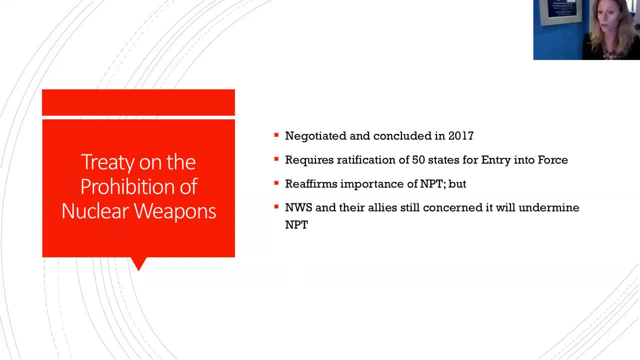 So one thing that I'd like to say at the outset that I think is helpful for framing this discussion is that when we use the term regime, we mean both sort of documents, things like treaties, negotiating bodies, so conferences and other groups of UN member states who talk about these issues and talk about how to strengthen them. 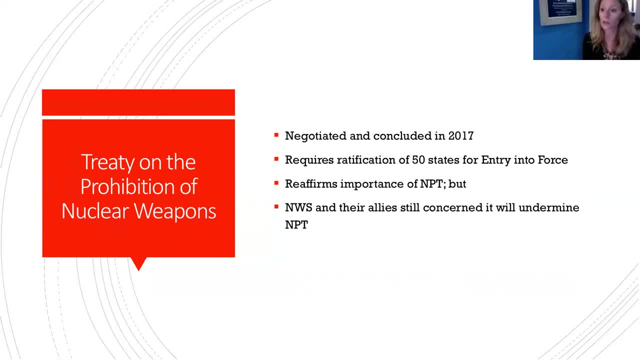 So one thing that I'd like to say at the outset that I think is helpful for framing this discussion is that when we use the term regime, we mean both sort of documents, things like treaties, negotiating bodies, so conferences and other groups of UN member states who talk about these issues and talk about how to strengthen them. 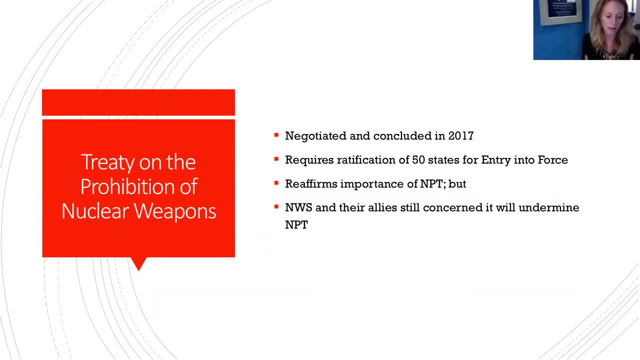 So one thing that I'd like to say at the outset that I think is helpful for framing this discussion is that when we use the term regime, we mean both sort of documents, things like treaties, negotiating bodies, so conferences and other groups of UN member states who talk about these issues and talk about how to strengthen them. 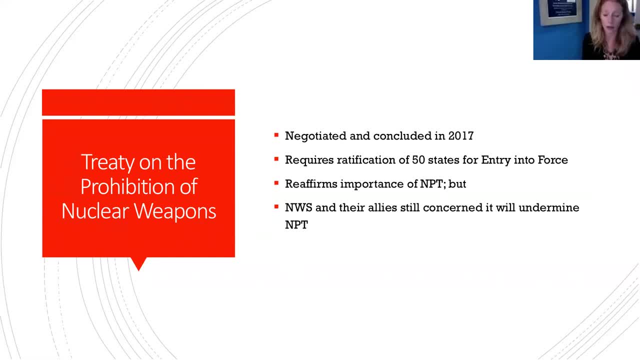 So one thing that I'd like to say at the outset that I think is helpful for framing this discussion is that when we use the term regime, we mean both sort of documents, things like treaties, negotiating bodies, so conferences and other groups of UN member states who talk about these issues and talk about how to strengthen them. 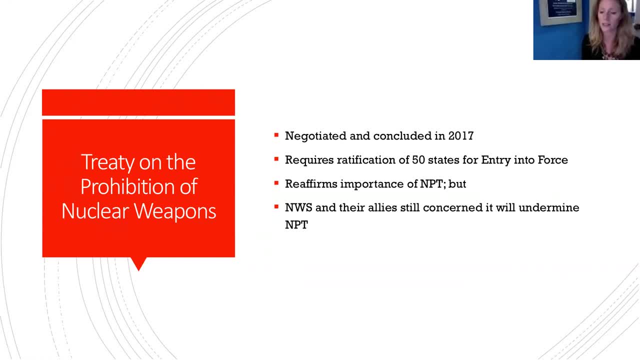 So one thing that I'd like to say at the outset that I think is helpful for framing this discussion is that when we use the term regime, we mean both sort of documents, things like treaties, negotiating bodies, so conferences and other groups of UN member states who talk about these issues and talk about how to strengthen them. 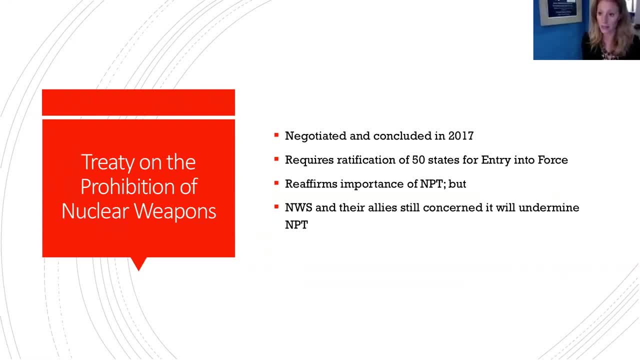 So one thing that I'd like to say at the outset that I think is helpful for framing this discussion is that when we use the term regime, we mean both sort of documents, things like treaties, negotiating bodies, so conferences and other groups of UN member states who talk about these issues and talk about how to strengthen them. 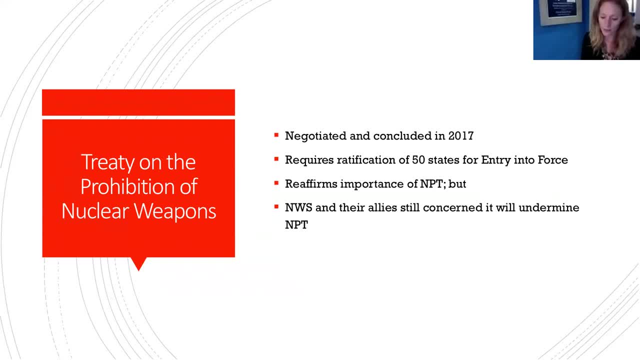 So one thing that I'd like to say at the outset that I think is helpful for framing this discussion is that when we use the term regime, we mean both sort of documents, things like treaties, negotiating bodies, so conferences and other groups of UN member states who talk about these issues and talk about how to strengthen them. 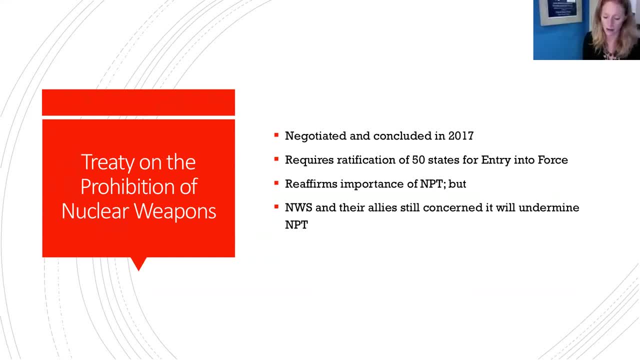 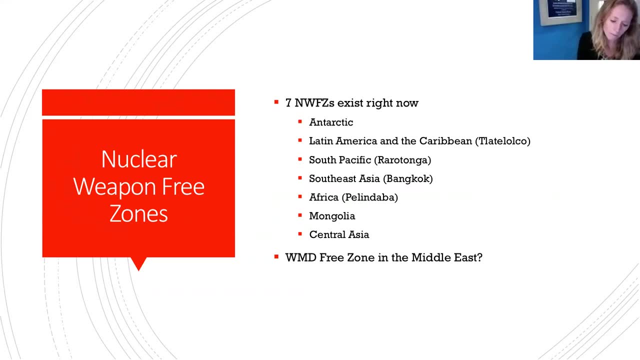 So one thing that I'd like to say at the outset that I think is helpful for framing this discussion is that when we use the term regime, we mean both sort of documents, things like treaties, negotiating bodies, so conferences and other groups of UN member states who talk about these issues and talk about how to strengthen them. 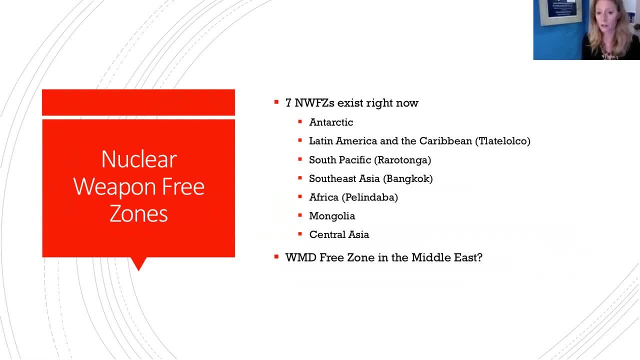 So one thing that I'd like to say at the outset that I think is helpful for framing this discussion is that when we use the term regime, we mean both sort of documents, things like treaties, negotiating bodies, so conferences and other groups of UN member states who talk about these issues and talk about how to strengthen them. 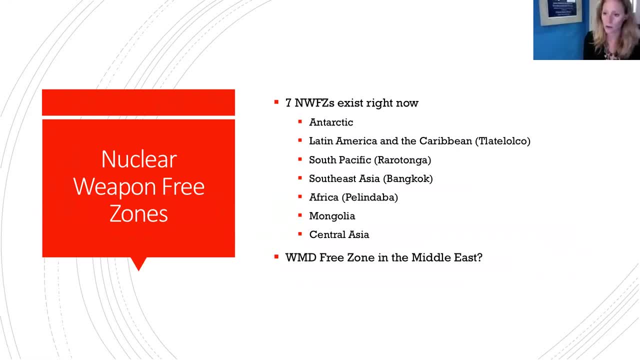 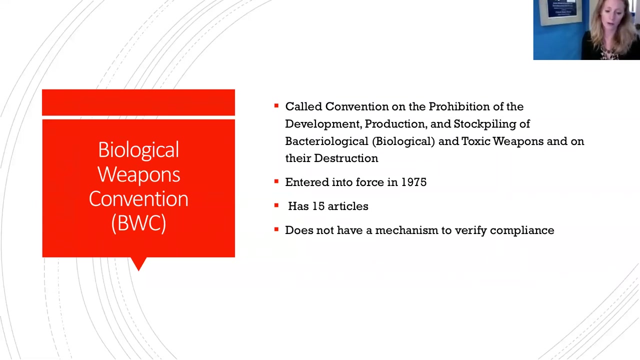 So one thing that I'd like to say at the outset that I think is helpful for framing this discussion is that when we use the term regime, we mean both sort of documents, things like treaties, negotiating bodies, so conferences and other groups of UN member states who talk about these issues and talk about how to strengthen them. 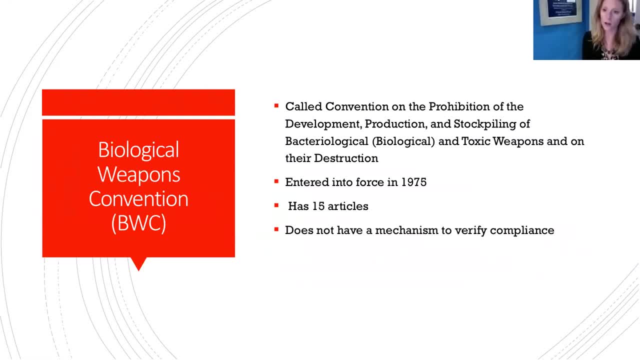 So one thing that I'd like to say at the outset that I think is helpful for framing this discussion is that when we use the term regime, we mean both sort of documents, things like treaties, negotiating bodies, so conferences and other groups of UN member states who talk about these issues and talk about how to strengthen them. 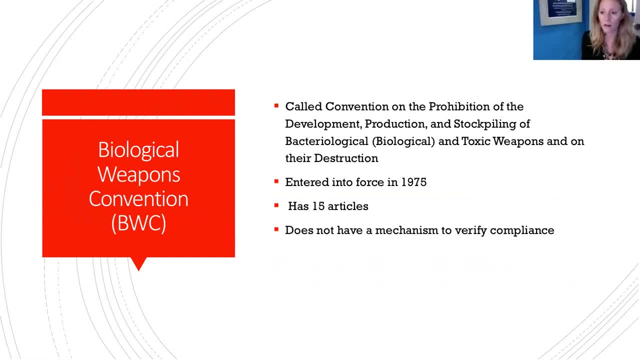 So one thing that I'd like to say at the outset that I think is helpful for framing this discussion is that when we use the term regime, we mean both sort of documents, things like treaties, negotiating bodies, so conferences and other groups of UN member states who talk about these issues and talk about how to strengthen them. 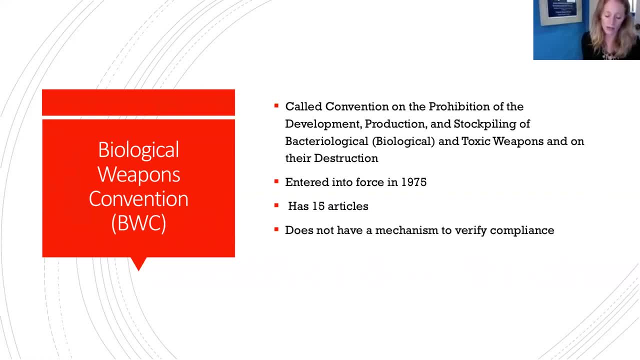 So one thing that I'd like to say at the outset that I think is helpful for framing this discussion is that when we use the term regime, we mean both sort of documents, things like treaties, negotiating bodies, so conferences and other groups of UN member states who talk about these issues and talk about how to strengthen them. 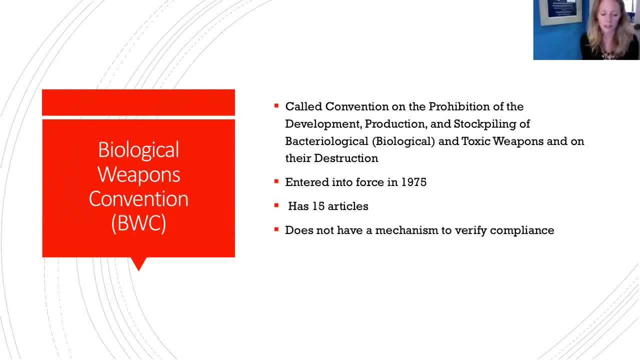 So one thing that I'd like to say at the outset that I think is helpful for framing this discussion is that when we use the term regime, we mean both sort of documents, things like treaties, negotiating bodies, so conferences and other groups of UN member states who talk about these issues and talk about how to strengthen them. 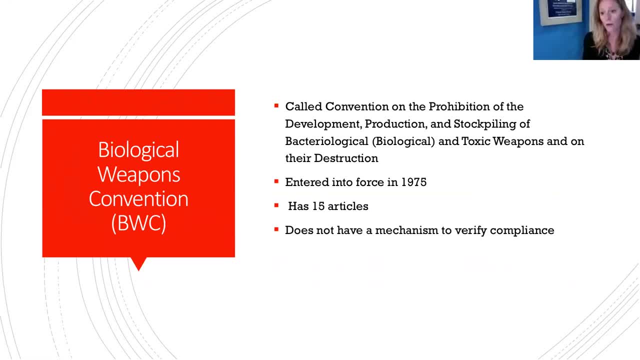 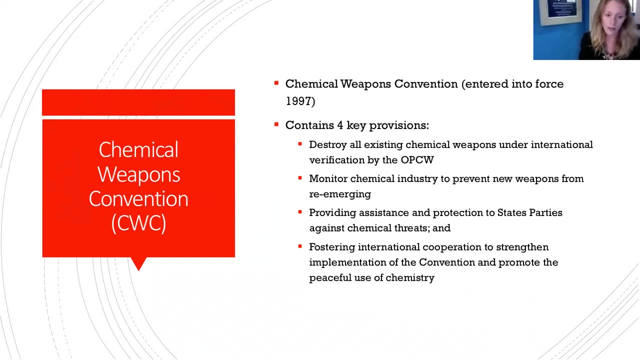 So one thing that I'd like to say at the outset that I think is helpful for framing this discussion is that when we use the term regime, we mean both sort of documents, things like treaties, negotiating bodies, so conferences and other groups of UN member states who talk about these issues and talk about how to strengthen them. 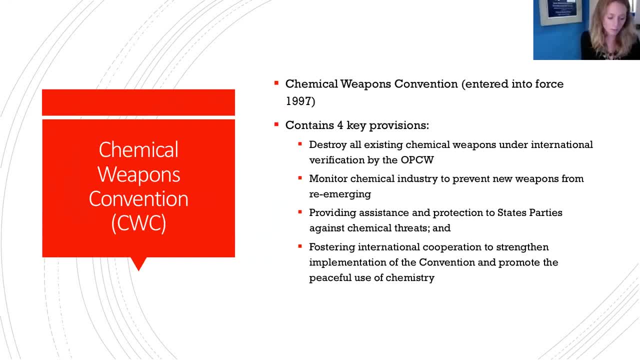 So one thing that I'd like to say at the outset that I think is helpful for framing this discussion is that when we use the term regime, we mean both sort of documents, things like treaties, negotiating bodies, so conferences and other groups of UN member states who talk about these issues and talk about how to strengthen them. 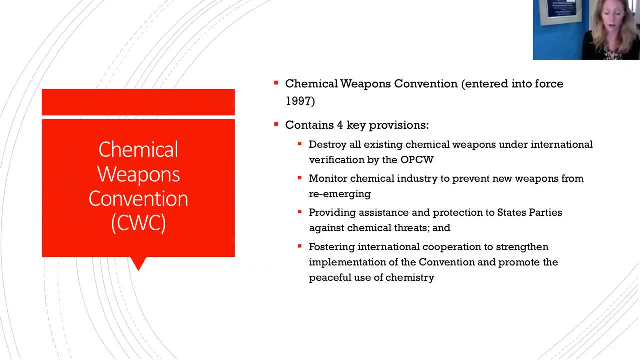 So one thing that I'd like to say at the outset that I think is helpful for framing this discussion is that when we use the term regime, we mean both sort of documents, things like treaties, negotiating bodies, so conferences and other groups of UN member states who talk about these issues and talk about how to strengthen them. 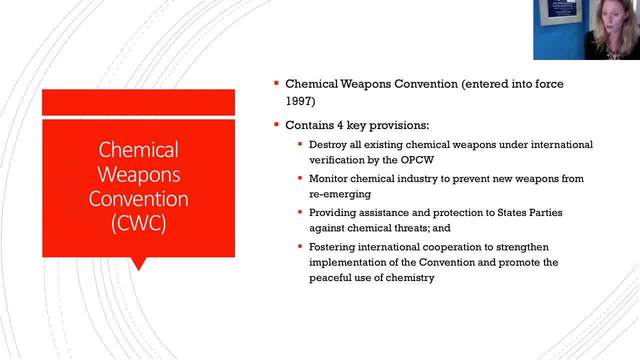 So one thing that I'd like to say at the outset that I think is helpful for framing this discussion is that when we use the term regime, we mean both sort of documents, things like treaties, negotiating bodies, so conferences and other groups of UN member states who talk about these issues and talk about how to strengthen them. 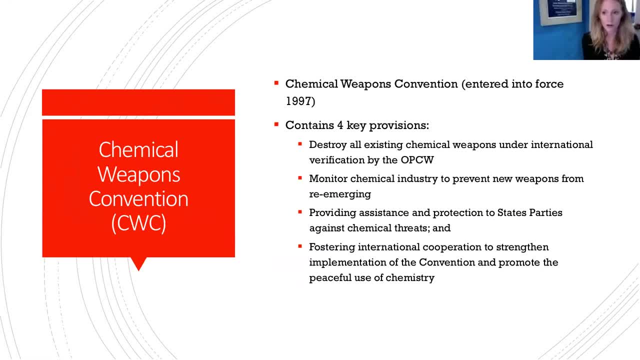 So one thing that I'd like to say at the outset that I think is helpful for framing this discussion is that when we use the term regime, we mean both sort of documents, things like treaties, negotiating bodies, so conferences and other groups of UN member states who talk about these issues and talk about how to strengthen them. 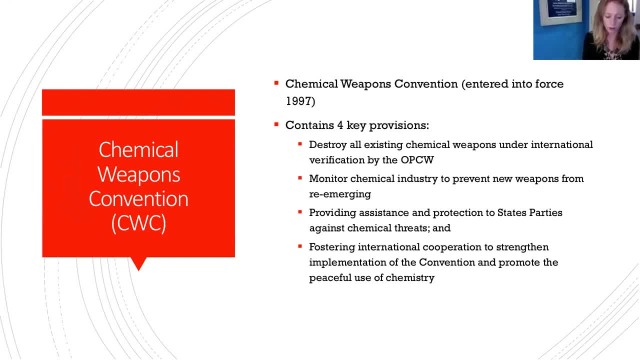 So one thing that I'd like to say at the outset that I think is helpful for framing this discussion is that when we use the term regime, we mean both sort of documents, things like treaties, negotiating bodies, so conferences and other groups of UN member states who talk about these issues and talk about how to strengthen them. 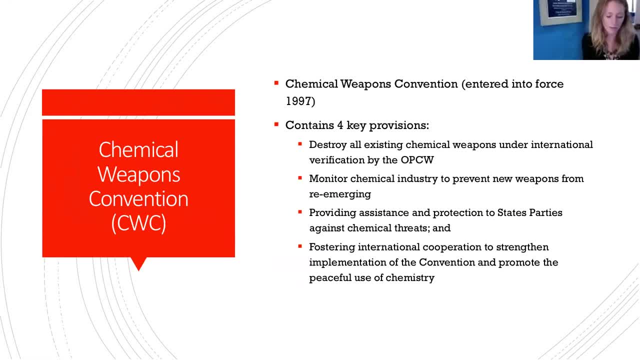 So one thing that I'd like to say at the outset that I think is helpful for framing this discussion is that when we use the term regime, we mean both sort of documents, things like treaties, negotiating bodies, so conferences and other groups of UN member states who talk about these issues and talk about how to strengthen them. 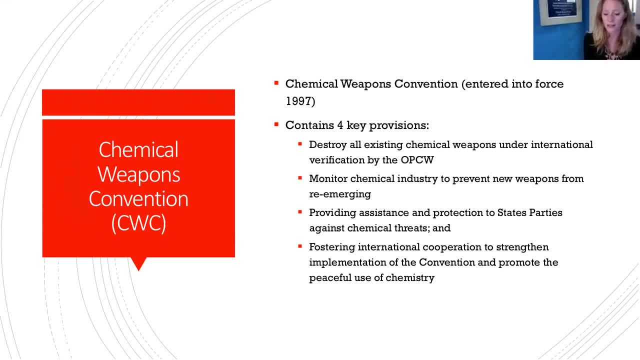 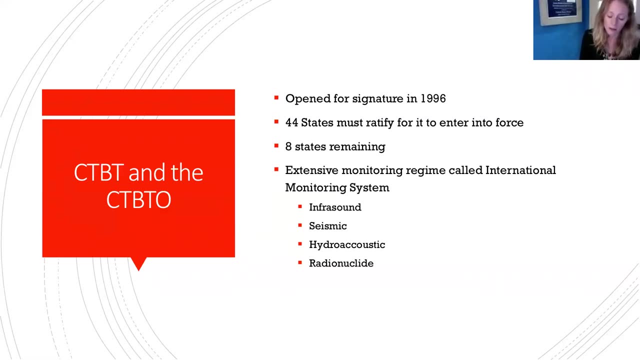 So one thing that I'd like to say at the outset that I think is helpful for framing this discussion is that when we use the term regime, we mean both sort of documents, things like treaties, negotiating bodies, so conferences and other groups of UN member states who talk about these issues and talk about how to strengthen them. 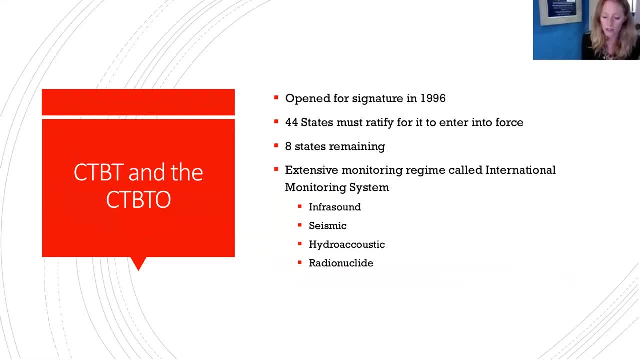 So one thing that I'd like to say at the outset that I think is helpful for framing this discussion is that when we use the term regime, we mean both sort of documents, things like treaties, negotiating bodies, so conferences and other groups of UN member states who talk about these issues and talk about how to strengthen them. 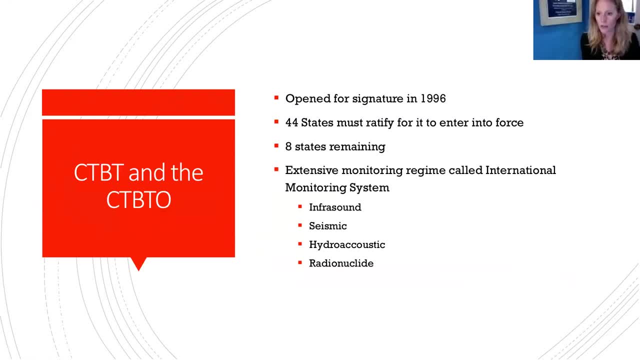 So one thing that I'd like to say at the outset that I think is helpful for framing this discussion is that when we use the term regime, we mean both sort of documents, things like treaties, negotiating bodies, so conferences and other groups of UN member states who talk about these issues and talk about how to strengthen them. 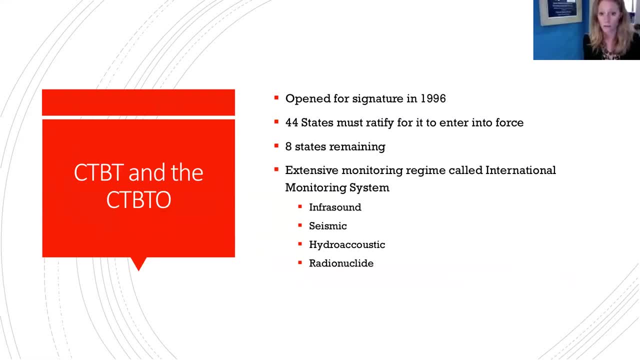 So one thing that I'd like to say at the outset that I think is helpful for framing this discussion is that when we use the term regime, we mean both sort of documents, things like treaties, negotiating bodies, so conferences and other groups of UN member states who talk about these issues and talk about how to strengthen them. 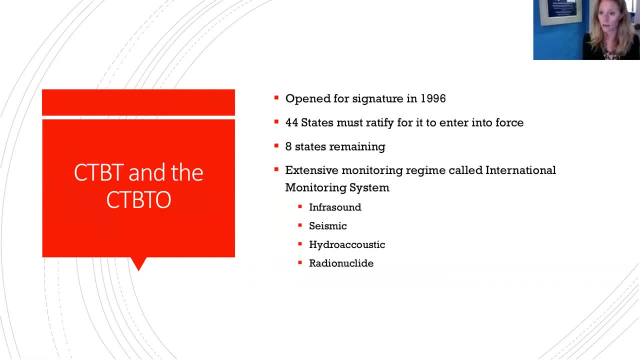 So one thing that I'd like to say at the outset that I think is helpful for framing this discussion is that when we use the term regime, we mean both sort of documents, things like treaties, negotiating bodies, so conferences and other groups of UN member states who talk about these issues and talk about how to strengthen them. 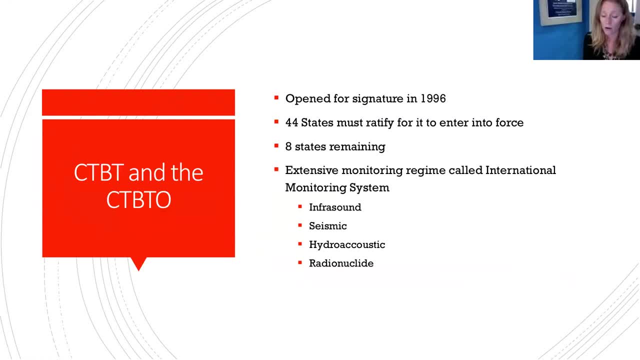 So one thing that I'd like to say at the outset that I think is helpful for framing this discussion is that when we use the term regime, we mean both sort of documents, things like treaties, negotiating bodies, so conferences and other groups of UN member states who talk about these issues and talk about how to strengthen them. 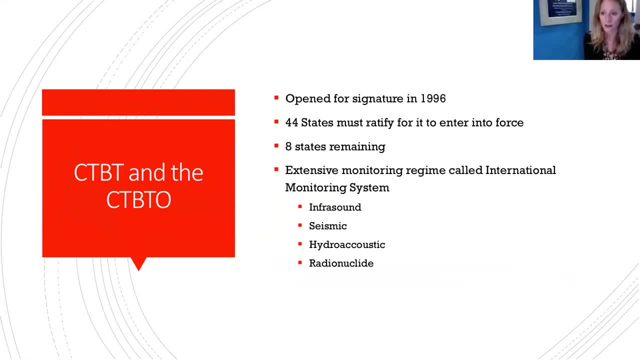 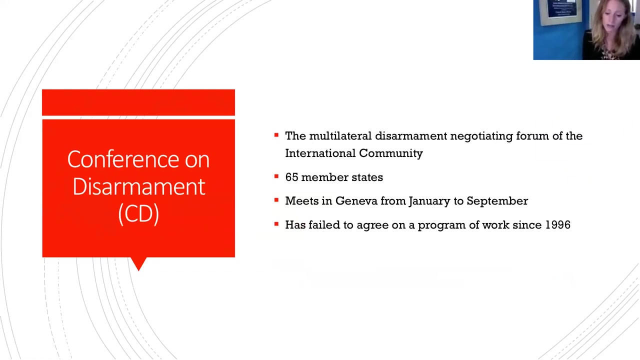 So one thing that I'd like to say at the outset that I think is helpful for framing this discussion is that when we use the term regime, we mean both sort of documents, things like treaties, negotiating bodies, so conferences and other groups of UN member states who talk about these issues and talk about how to strengthen them. 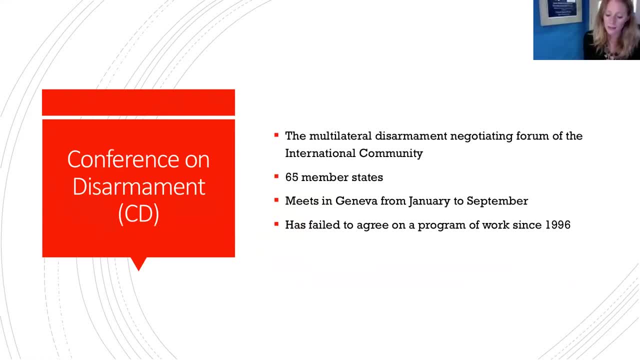 So one thing that I'd like to say at the outset that I think is helpful for framing this discussion is that when we use the term regime, we mean both sort of documents, things like treaties, negotiating bodies, so conferences and other groups of UN member states who talk about these issues and talk about how to strengthen them. 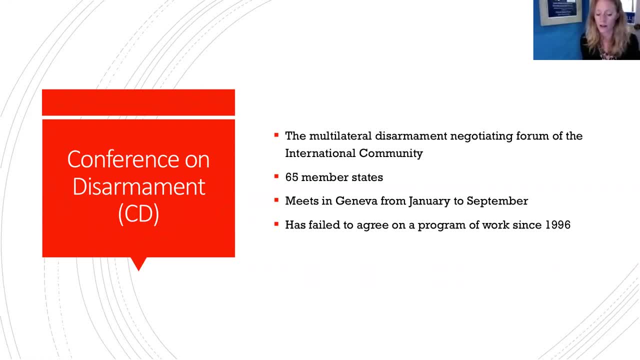 So one thing that I'd like to say at the outset that I think is helpful for framing this discussion is that when we use the term regime, we mean both sort of documents, things like treaties, negotiating bodies, so conferences and other groups of UN member states who talk about these issues and talk about how to strengthen them. 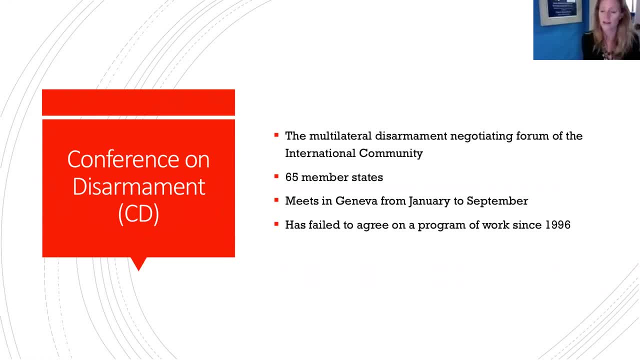 So one thing that I'd like to say at the outset that I think is helpful for framing this discussion is that when we use the term regime, we mean both sort of documents, things like treaties, negotiating bodies, so conferences and other groups of UN member states who talk about these issues and talk about how to strengthen them. 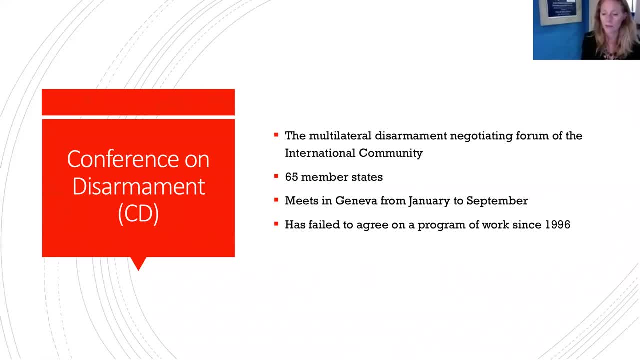 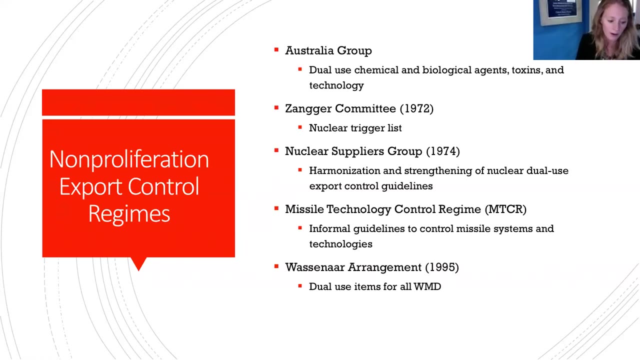 So one thing that I'd like to say at the outset that I think is helpful for framing this discussion is that when we use the term regime, we mean both sort of documents, things like treaties, negotiating bodies, so conferences and other groups of UN member states who talk about these issues and talk about how to strengthen them. 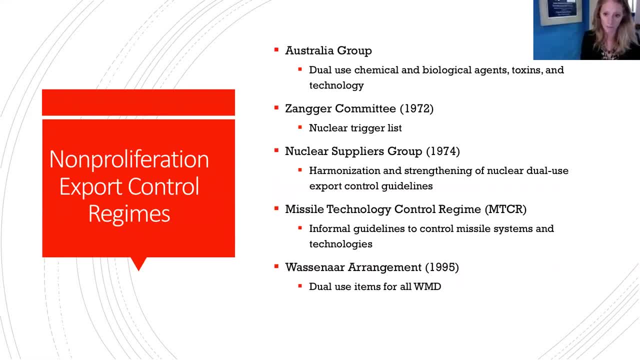 So one thing that I'd like to say at the outset that I think is helpful for framing this discussion is that when we use the term regime, we mean both sort of documents, things like treaties, negotiating bodies, so conferences and other groups of UN member states who talk about these issues and talk about how to strengthen them. 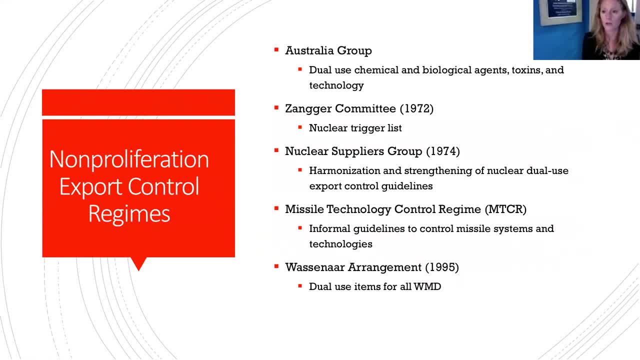 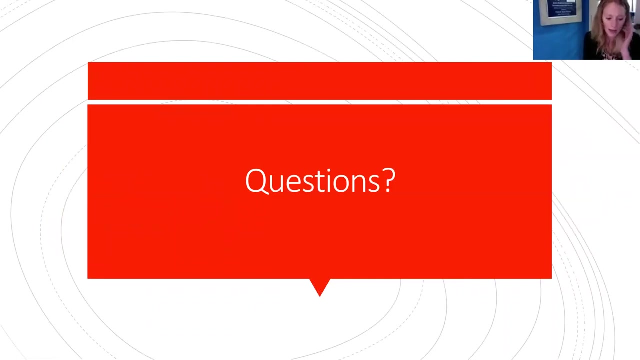 So one thing that I'd like to say at the outset that I think is helpful for framing this discussion is that when we use the term regime, we mean both sort of documents, things like treaties, negotiating bodies, so conferences and other groups of UN member states who talk about these issues and talk about how to strengthen them. 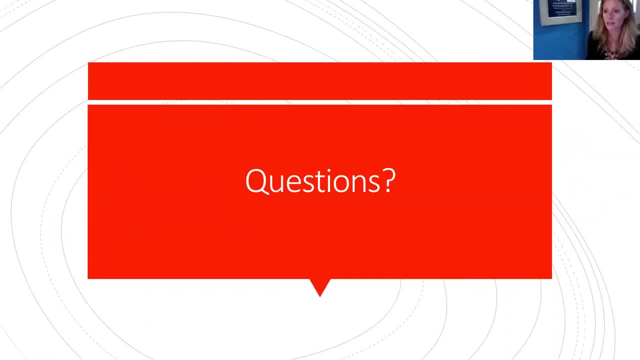 So one thing that I'd like to say at the outset that I think is helpful for framing this discussion is that when we use the term regime, we mean both sort of documents, things like treaties, negotiating bodies, so conferences and other groups of UN member states who talk about these issues and talk about how to strengthen them. 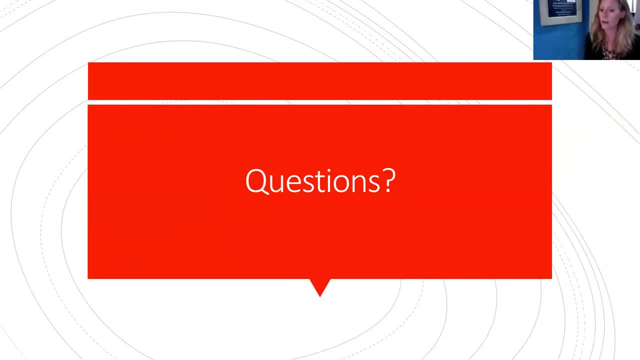 So one thing that I'd like to say at the outset that I think is helpful for framing this discussion is that when we use the term regime, we mean both sort of documents, things like treaties, negotiating bodies, so conferences and other groups of UN member states who talk about these issues and talk about how to strengthen them. 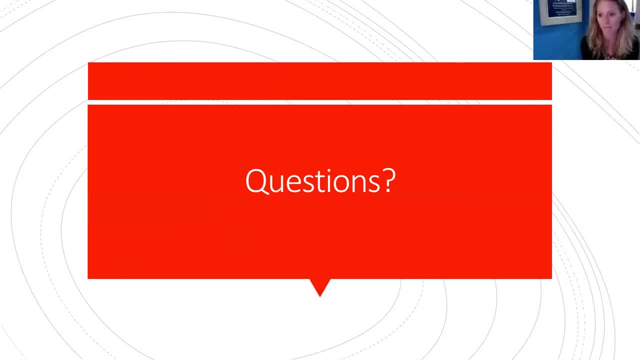 So one thing that I'd like to say at the outset that I think is helpful for framing this discussion is that when we use the term regime, we mean both sort of documents, things like treaties, negotiating bodies, so conferences and other groups of UN member states who talk about these issues and talk about how to strengthen them. 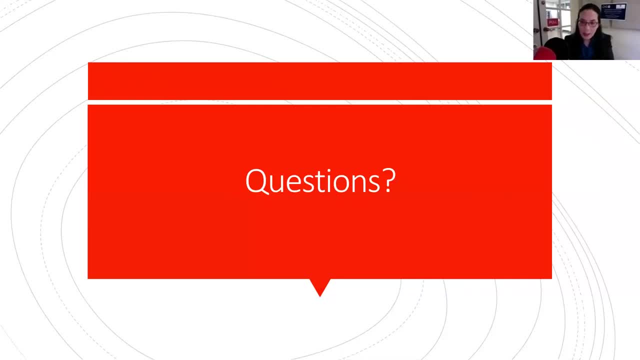 So one thing that I'd like to say at the outset that I think is helpful for framing this discussion is that when we use the term regime, we mean both sort of documents, things like treaties, negotiating bodies, so conferences and other groups of UN member states who talk about these issues and talk about how to strengthen them. 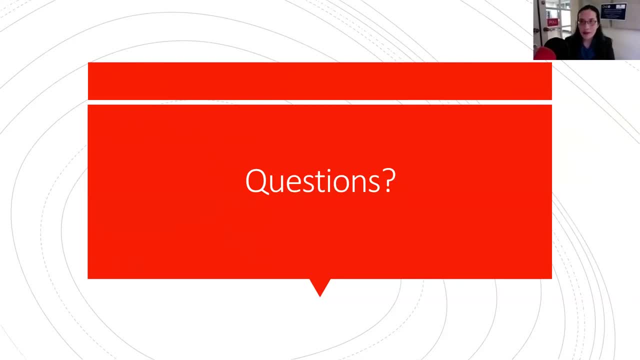 So one thing that I'd like to say at the outset that I think is helpful for framing this discussion is that when we use the term regime, we mean both sort of documents, things like treaties, negotiating bodies, so conferences and other groups of UN member states who talk about these issues and talk about how to strengthen them. 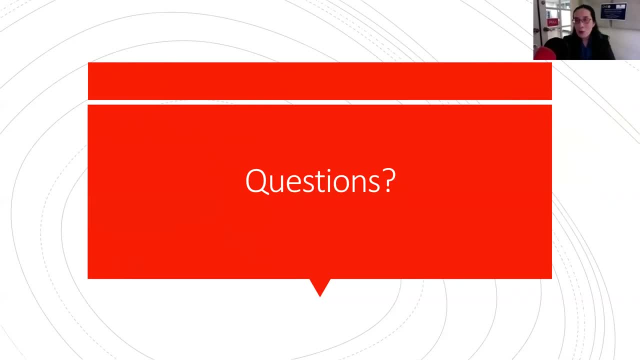 So one thing that I'd like to say at the outset that I think is helpful for framing this discussion is that when we use the term regime, we mean both sort of documents, things like treaties, negotiating bodies, so conferences and other groups of UN member states who talk about these issues and talk about how to strengthen them. 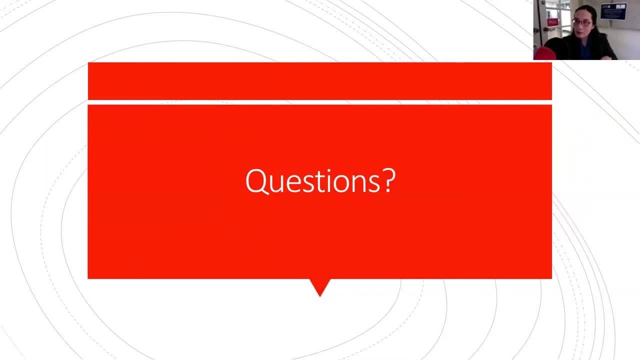 So one thing that I'd like to say at the outset that I think is helpful for framing this discussion is that when we use the term regime, we mean both sort of documents, things like treaties, negotiating bodies, so conferences and other groups of UN member states who talk about these issues and talk about how to strengthen them. 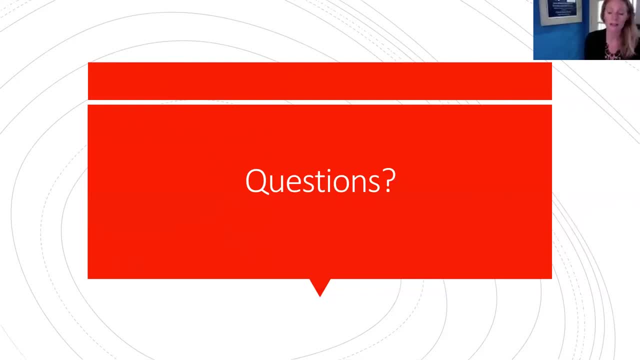 So one thing that I'd like to say at the outset that I think is helpful for framing this discussion is that when we use the term regime, we mean both sort of documents, things like treaties, negotiating bodies, so conferences and other groups of UN member states who talk about these issues and talk about how to strengthen them. 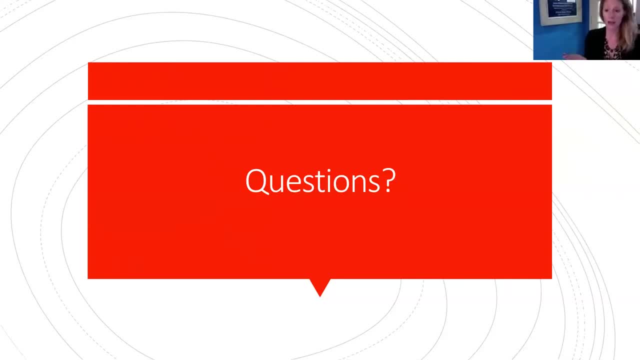 So one thing that I'd like to say at the outset that I think is helpful for framing this discussion is that when we use the term regime, we mean both sort of documents, things like treaties, negotiating bodies, so conferences and other groups of UN member states who talk about these issues and talk about how to strengthen them. 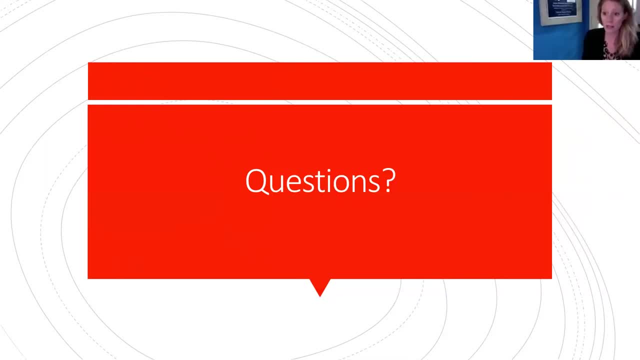 So one thing that I'd like to say at the outset that I think is helpful for framing this discussion is that when we use the term regime, we mean both sort of documents, things like treaties, negotiating bodies, so conferences and other groups of UN member states who talk about these issues and talk about how to strengthen them. 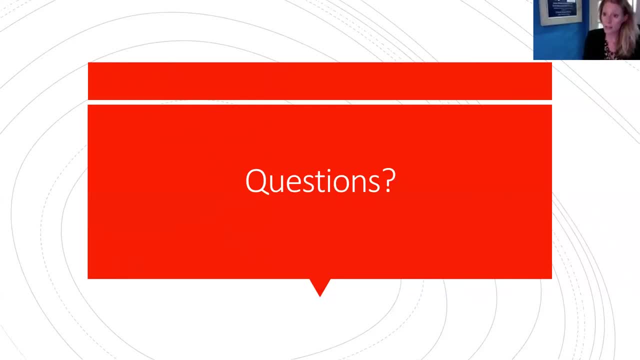 So one thing that I'd like to say at the outset that I think is helpful for framing this discussion is that when we use the term regime, we mean both sort of documents, things like treaties, negotiating bodies, so conferences and other groups of UN member states who talk about these issues and talk about how to strengthen them. 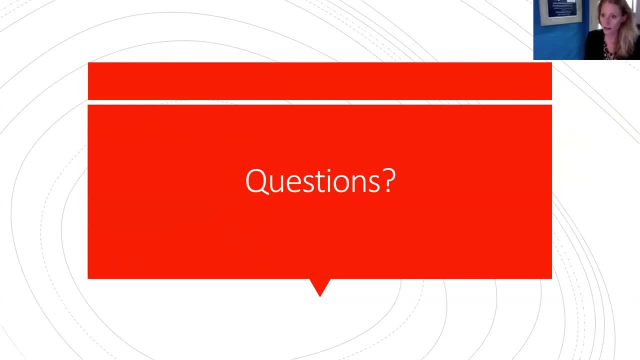 So one thing that I'd like to say at the outset that I think is helpful for framing this discussion is that when we use the term regime, we mean both sort of documents, things like treaties, negotiating bodies, so conferences and other groups of UN member states who talk about these issues and talk about how to strengthen them. 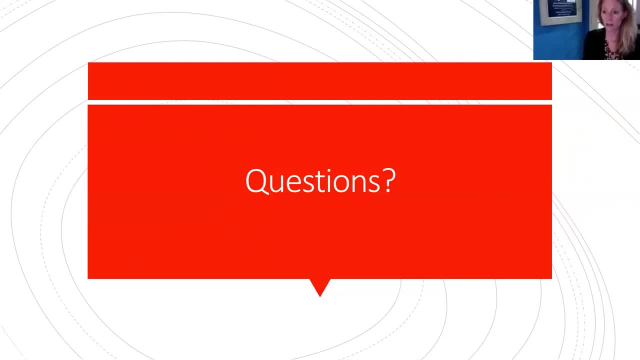 So one thing that I'd like to say at the outset that I think is helpful for framing this discussion is that when we use the term regime, we mean both sort of documents, things like treaties, negotiating bodies, so conferences and other groups of UN member states who talk about these issues and talk about how to strengthen them. 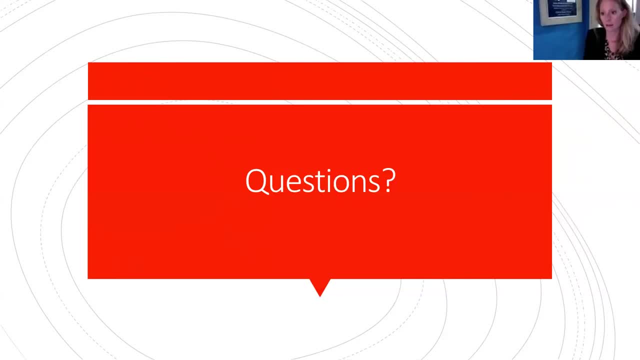 So one thing that I'd like to say at the outset that I think is helpful for framing this discussion is that when we use the term regime, we mean both sort of documents, things like treaties, negotiating bodies, so conferences and other groups of UN member states who talk about these issues and talk about how to strengthen them. 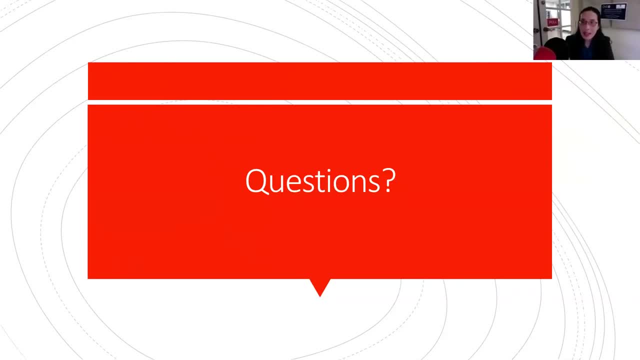 So one thing that I'd like to say at the outset that I think is helpful for framing this discussion is that when we use the term regime, we mean both sort of documents, things like treaties, negotiating bodies, so conferences and other groups of UN member states who talk about these issues and talk about how to strengthen them. 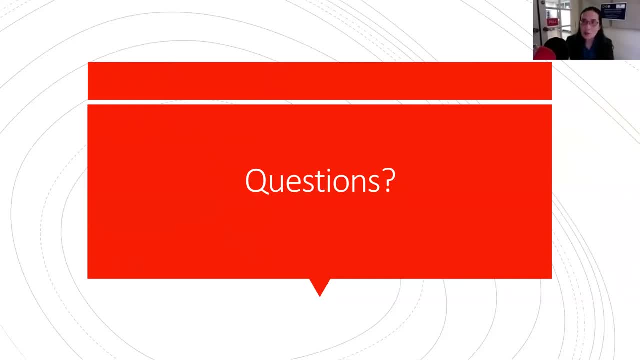 So one thing that I'd like to say at the outset that I think is helpful for framing this discussion is that when we use the term regime, we mean both sort of documents, things like treaties, negotiating bodies, so conferences and other groups of UN member states who talk about these issues and talk about how to strengthen them. 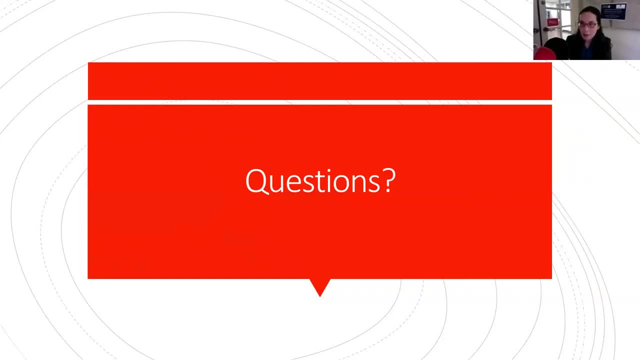 So one thing that I'd like to say at the outset that I think is helpful for framing this discussion is that when we use the term regime, we mean both sort of documents, things like treaties, negotiating bodies, so conferences and other groups of UN member states who talk about these issues and talk about how to strengthen them. 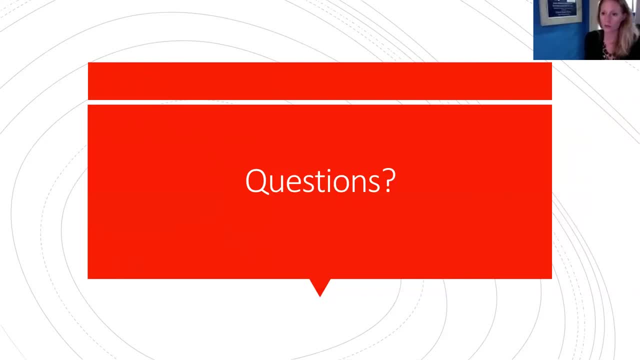 So one thing that I'd like to say at the outset that I think is helpful for framing this discussion is that when we use the term regime, we mean both sort of documents, things like treaties, negotiating bodies, so conferences and other groups of UN member states who talk about these issues and talk about how to strengthen them. 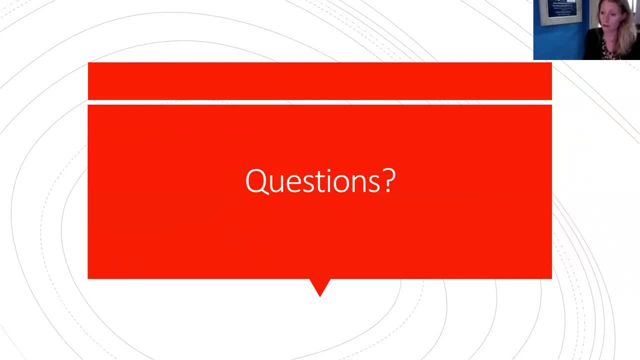 So one thing that I'd like to say at the outset that I think is helpful for framing this discussion is that when we use the term regime, we mean both sort of documents, things like treaties, negotiating bodies, so conferences and other groups of UN member states who talk about these issues and talk about how to strengthen them. 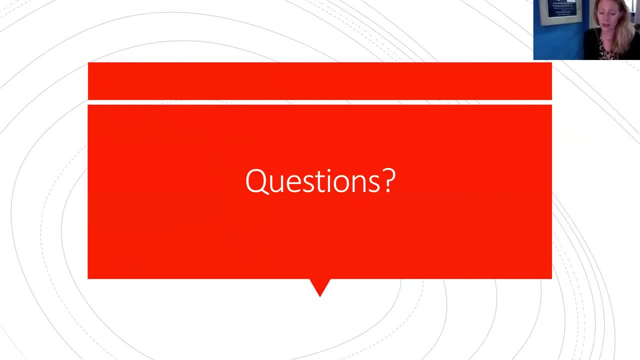 So one thing that I'd like to say at the outset that I think is helpful for framing this discussion is that when we use the term regime, we mean both sort of documents, things like treaties, negotiating bodies, so conferences and other groups of UN member states who talk about these issues and talk about how to strengthen them. 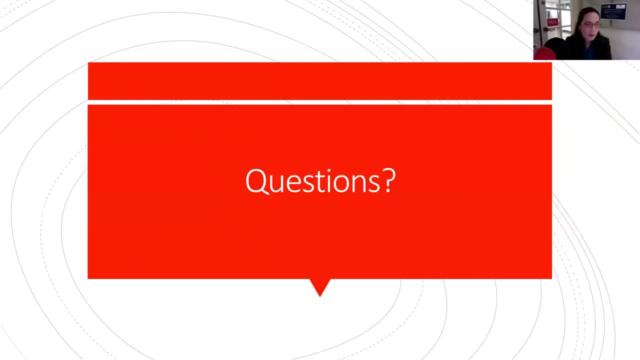 So one thing that I'd like to say at the outset that I think is helpful for framing this discussion is that when we use the term regime, we mean both sort of documents, things like treaties, negotiating bodies, so conferences and other groups of UN member states who talk about these issues and talk about how to strengthen them. 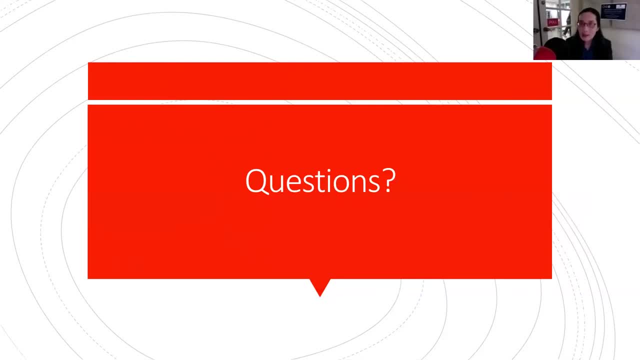 So one thing that I'd like to say at the outset that I think is helpful for framing this discussion is that when we use the term regime, we mean both sort of documents, things like treaties, negotiating bodies, so conferences and other groups of UN member states who talk about these issues and talk about how to strengthen them. 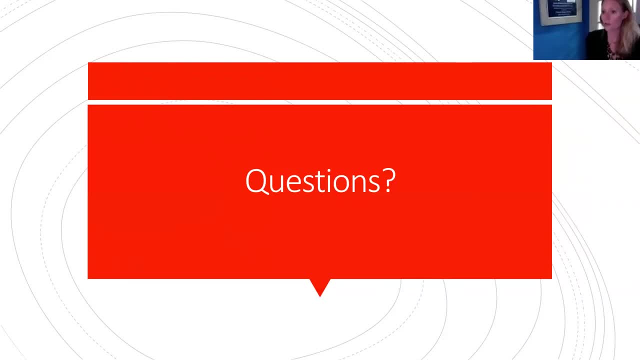 So one thing that I'd like to say at the outset that I think is helpful for framing this discussion is that when we use the term regime, we mean both sort of documents, things like treaties, negotiating bodies, so conferences and other groups of UN member states who talk about these issues and talk about how to strengthen them. 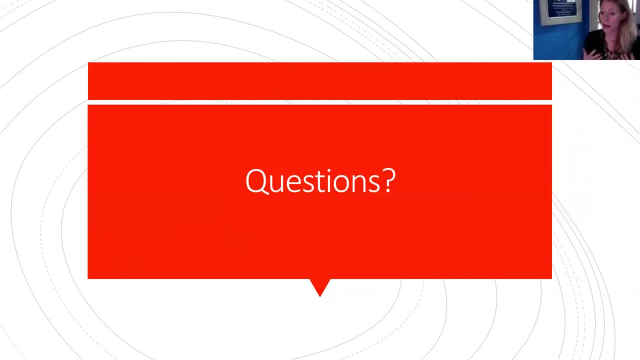 So one thing that I'd like to say at the outset that I think is helpful for framing this discussion is that when we use the term regime, we mean both sort of documents, things like treaties, negotiating bodies, so conferences and other groups of UN member states who talk about these issues and talk about how to strengthen them. 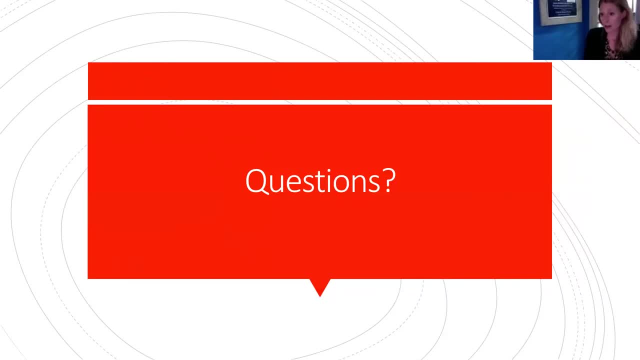 So one thing that I'd like to say at the outset that I think is helpful for framing this discussion is that when we use the term regime, we mean both sort of documents, things like treaties, negotiating bodies, so conferences and other groups of UN member states who talk about these issues and talk about how to strengthen them. 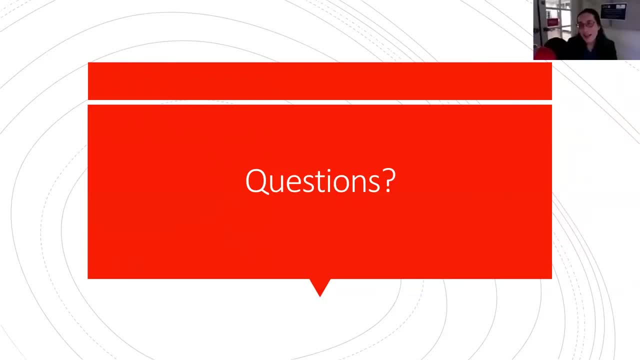 So one thing that I'd like to say at the outset that I think is helpful for framing this discussion is that when we use the term regime, we mean both sort of documents, things like treaties, negotiating bodies, so conferences and other groups of UN member states who talk about these issues and talk about how to strengthen them. 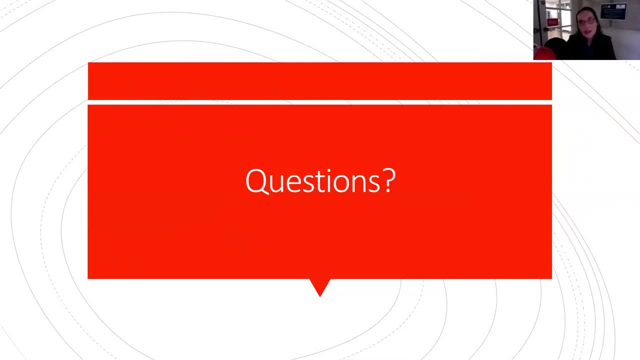 So one thing that I'd like to say at the outset that I think is helpful for framing this discussion is that when we use the term regime, we mean both sort of documents, things like treaties, negotiating bodies, so conferences and other groups of UN member states who talk about these issues and talk about how to strengthen them. 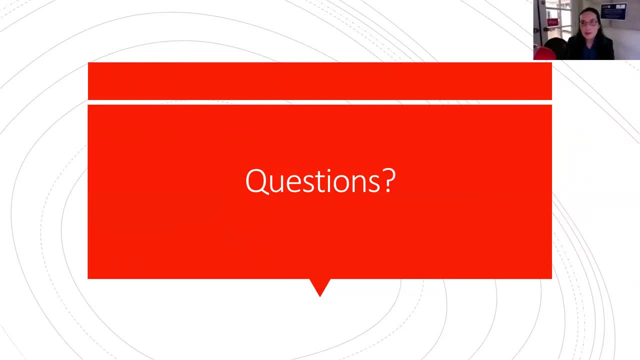 So one thing that I'd like to say at the outset that I think is helpful for framing this discussion is that when we use the term regime, we mean both sort of documents, things like treaties, negotiating bodies, so conferences and other groups of UN member states who talk about these issues and talk about how to strengthen them. 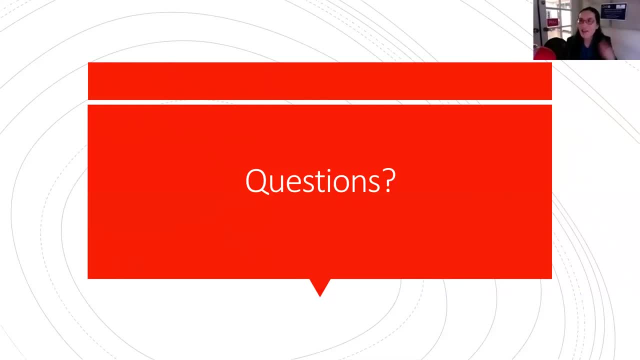 So one thing that I'd like to say at the outset that I think is helpful for framing this discussion is that when we use the term regime, we mean both sort of documents, things like treaties, negotiating bodies, so conferences and other groups of UN member states who talk about these issues and talk about how to strengthen them. 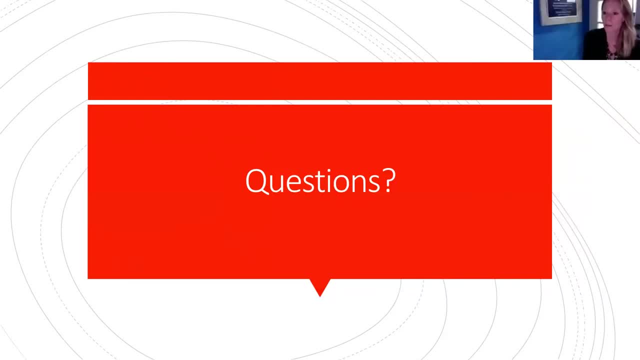 So one thing that I'd like to say at the outset that I think is helpful for framing this discussion is that when we use the term regime, we mean both sort of documents, things like treaties, negotiating bodies, so conferences and other groups of UN member states who talk about these issues and talk about how to strengthen them. 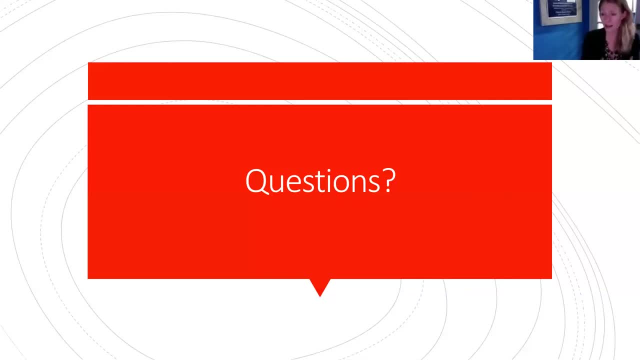 So one thing that I'd like to say at the outset that I think is helpful for framing this discussion is that when we use the term regime, we mean both sort of documents, things like treaties, negotiating bodies, so conferences and other groups of UN member states who talk about these issues and talk about how to strengthen them. 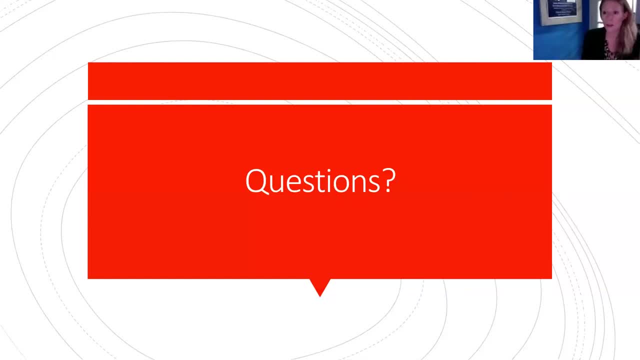 So one thing that I'd like to say at the outset that I think is helpful for framing this discussion is that when we use the term regime, we mean both sort of documents, things like treaties, negotiating bodies, so conferences and other groups of UN member states who talk about these issues and talk about how to strengthen them. 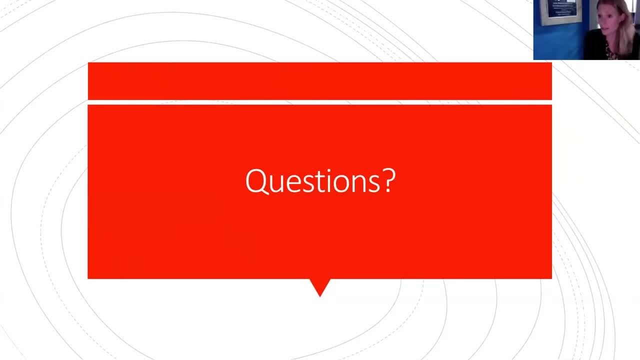 So one thing that I'd like to say at the outset that I think is helpful for framing this discussion is that when we use the term regime, we mean both sort of documents, things like treaties, negotiating bodies, so conferences and other groups of UN member states who talk about these issues and talk about how to strengthen them. 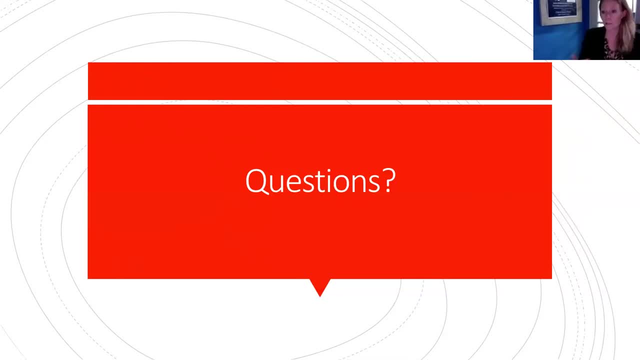 So one thing that I'd like to say at the outset that I think is helpful for framing this discussion is that when we use the term regime, we mean both sort of documents, things like treaties, negotiating bodies, so conferences and other groups of UN member states who talk about these issues and talk about how to strengthen them. 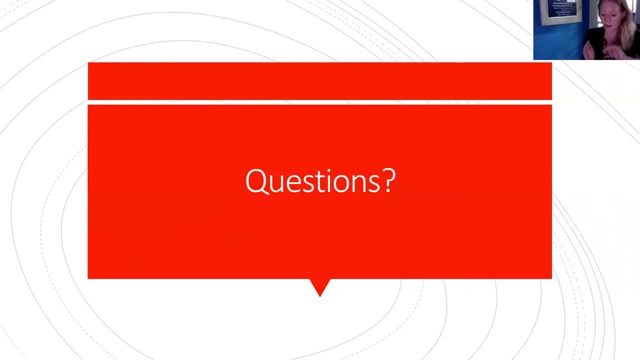 So one thing that I'd like to say at the outset that I think is helpful for framing this discussion is that when we use the term regime, we mean both sort of documents, things like treaties, negotiating bodies, so conferences and other groups of UN member states who talk about these issues and talk about how to strengthen them. 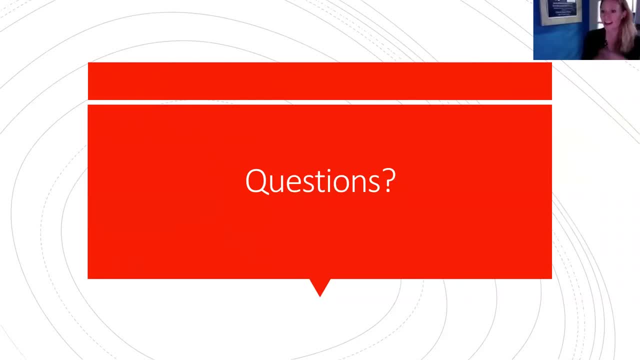 So one thing that I'd like to say at the outset that I think is helpful for framing this discussion is that when we use the term regime, we mean both sort of documents, things like treaties, negotiating bodies, so conferences and other groups of UN member states who talk about these issues and talk about how to strengthen them. 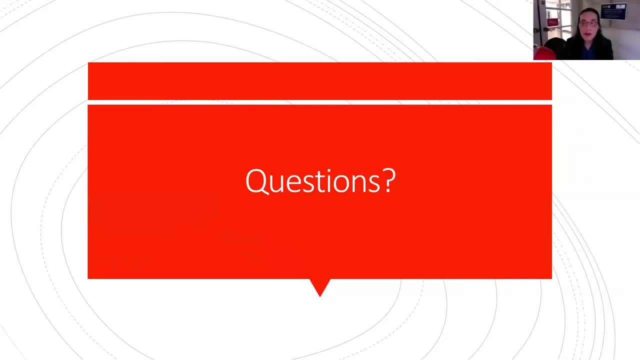 So one thing that I'd like to say at the outset that I think is helpful for framing this discussion is that when we use the term regime, we mean both sort of documents, things like treaties, negotiating bodies, so conferences and other groups of UN member states who talk about these issues and talk about how to strengthen them.